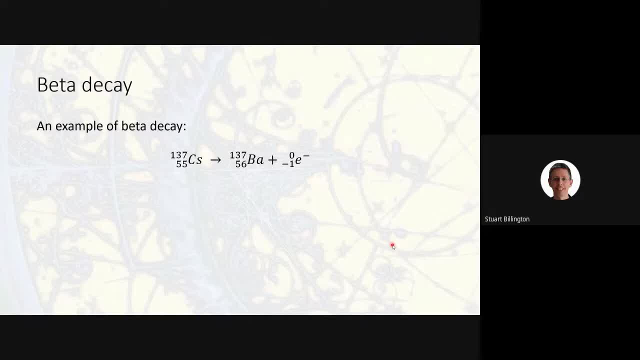 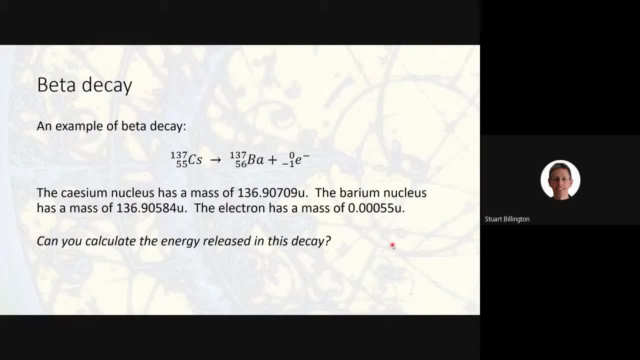 got a calculator with you. There is the mass of the cesium nucleus and the mass of the barium nucleus and the mass of the electron, all in atomic mass units. And what I would like you to do for me please on your calculator now I'll give you three minutes- is: could you please work? 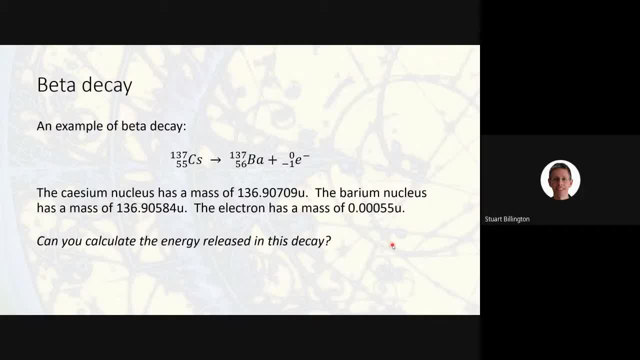 out how much energy is released when the cesium turns into the barium and the electron. So start off with that, And then I'll give you three minutes to work out how much energy is released when the cesium turns into the barium and the electron. So start off with a mass difference. 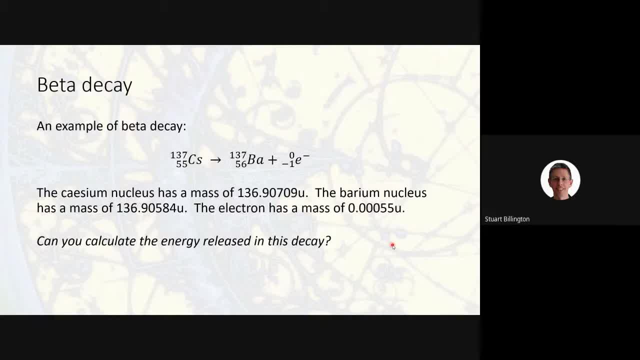 calculation and then turn your atomic mass units into kilograms using the conversion factor, which you may need to look up in your textbook or on your phone. And then you need to convert the kilograms into energy using Einstein's: E equals mc squared, And that'll give you an answer. 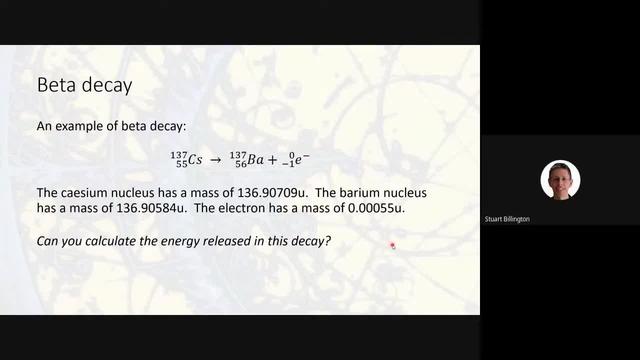 in joules, And then I need you to convert your joules into electron volts or mega electron volts, please, using the elementary charge as your conversion factor. So I'm going to give you three minutes. I'd like an energy, please for that decay. 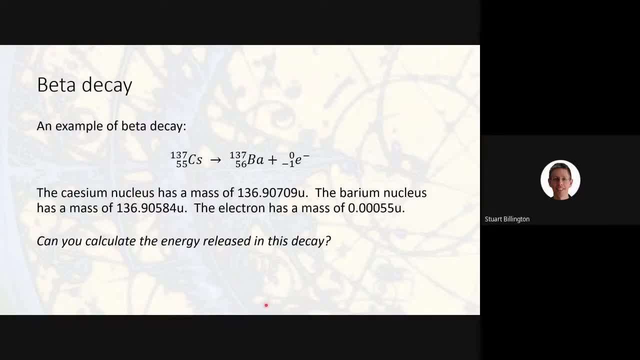 NASA Jet Propulsion Laboratory, California Institute of Technology. you, you, you, you. okay, I'll start the calculation on the screen. so you should have got that. the mass difference was uh, 7.0 times 10 to the minus four. make sure you don't lose a significant figure. make sure that your zero is still after the seven. 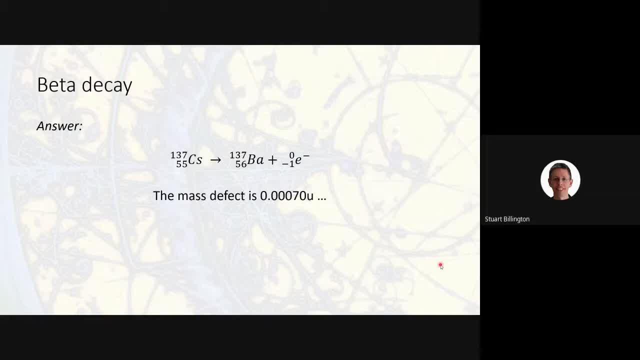 so that's an atomic mass unit. and then you need to remember that every atomic mass unit is 1.6605 times 10 to the minus 27 kilograms. so that allows you to turn your mass difference into kilograms. and then your formula for turning kilograms into energy is to multiply by c squared. 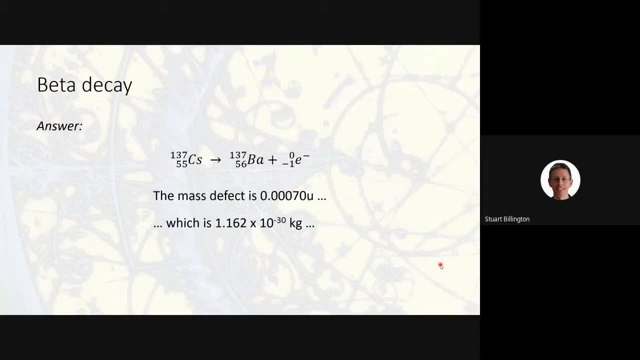 and c is three times 10 to the eight. so you need to square that and that gives you your energy in joules. and then you need to remember that every joule is 1.6 something times 10 to the minus 19. sorry, 1.6 times 10 to the minus 19, joules is: 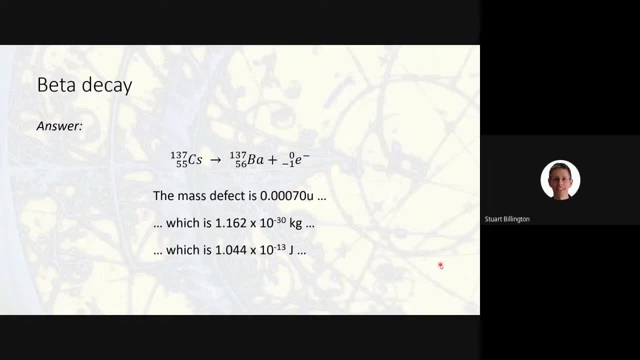 one electron volt. so if you divide that by 1.6 times 10 to the minus 19, you'll turn your joules into electron volts, and if you take out a factor of 10 to the six, you'll get it in mega electrons volts. so remember that what we said when we were doing the energy. 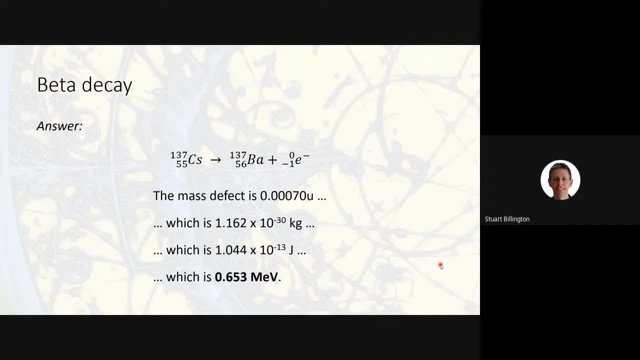 lesson was that anything in um a few mega electron volts was an appropriate number. so that's half a mega electron volt- near enough there. so that's an appropriate answer for a nuclear energy calculation. okay, so now that you're able to do that calculation, you know something that you didn't. 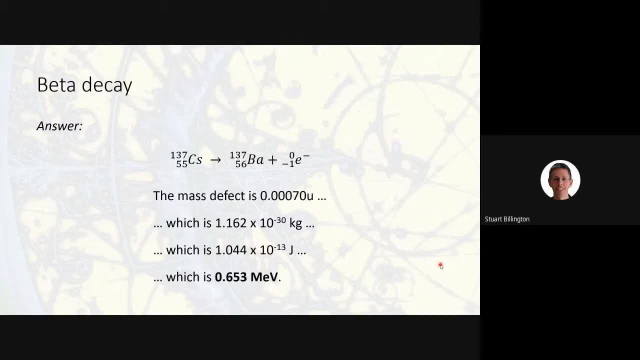 know when you were at gcse, which is that, alongside the emission of the electron, there is a release into the universe of some energy. and the question is now: where does the energy go? well, energy isn't really this mysterious, uh, substance that exists in its own rights. 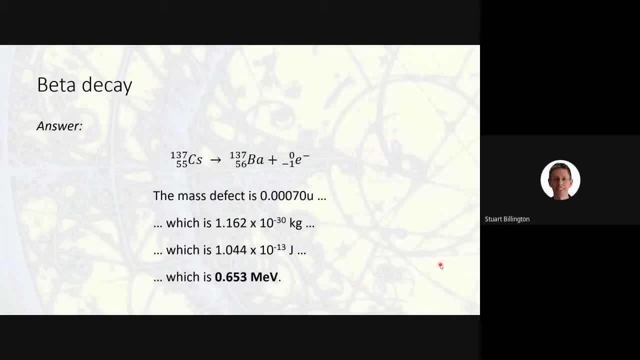 energy will be associated with objects and in this case, um, it's reasonable to assume that the barium and the electron have got the energy because, um, we don't detect any emission of gamma rays or anything like that, so we don't think there's any electromagnetic emission. so the only place that the energy can be is with the particles. 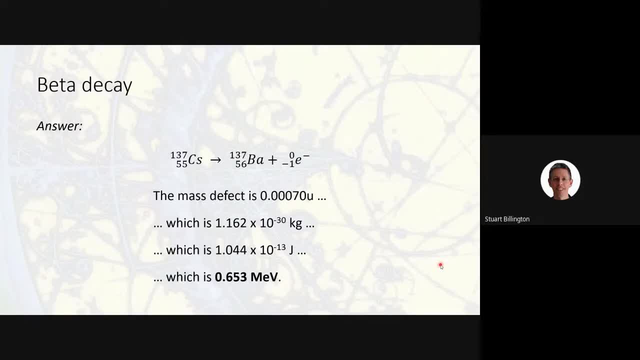 so we expect that the barium and the electron will have 0.653 mega electron volts of kinetic energy that the cesium didn't have. so if you consider that the cesium was stationary at the beginning, we expect the barium and the beta particle to be moving. 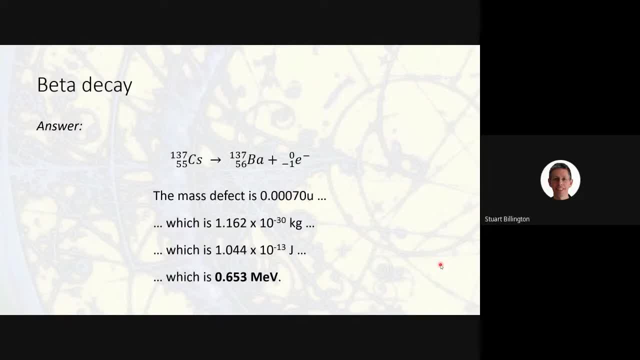 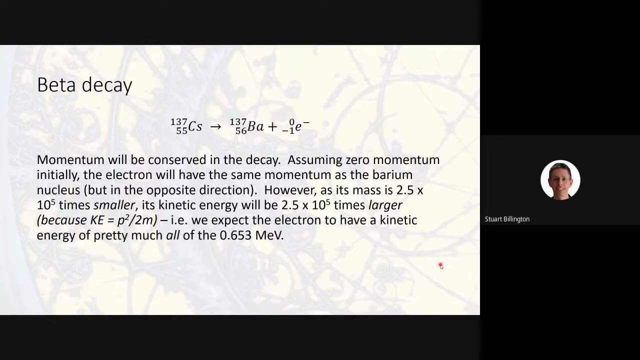 and, of course, we know the beta particles moving, because it's emitted and we, uh, detect it traveling through the air outside of the cesium nucleus. okay, so let's just do some more physics. so you know about momentum. so the cesium doesn't have any momentum. 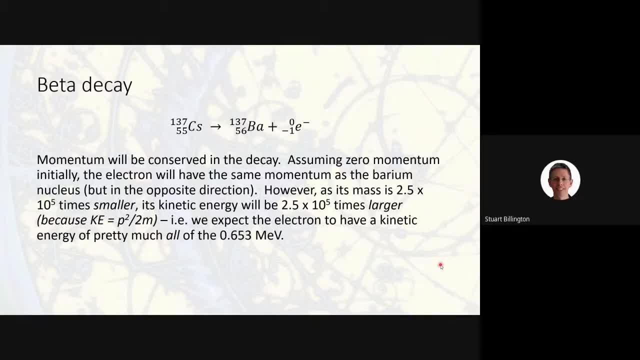 and when it decays, the barium and the electron between them must still have a net zero amount of momentum, and this is an explosion type um situation: the barium is going to go one way, the electron is going to go the other way and they'll have equal amounts of. 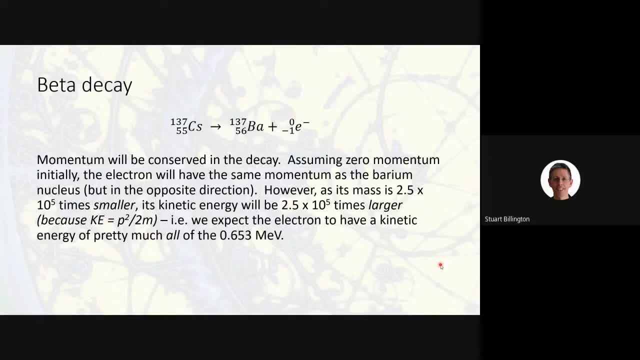 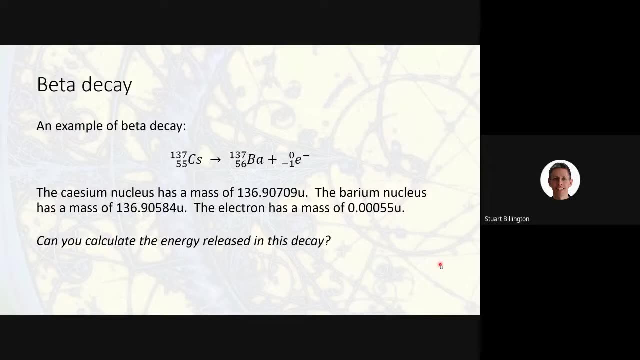 momentum, but one will be positive and one will be negative and when it adds up it'll sum to zero. so if we just consider the masses of the barium and the electron, if you just look back to the calculation that we- the numbers we just have had, 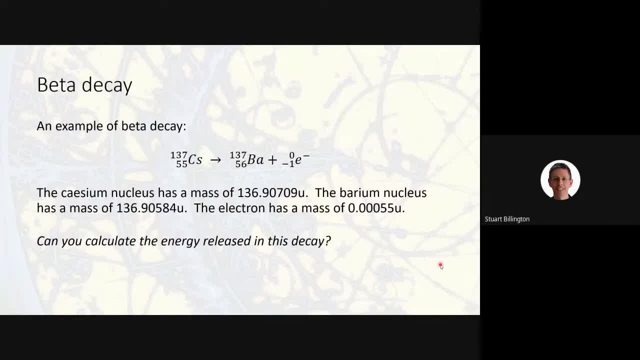 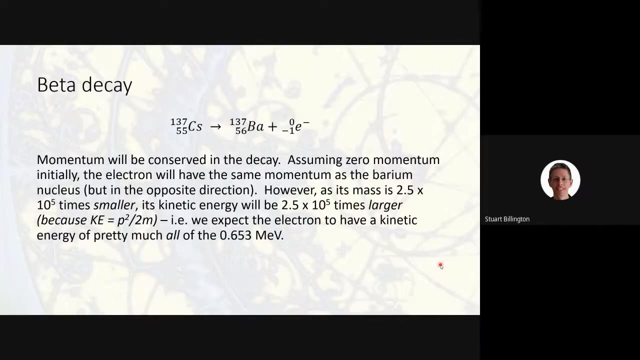 you consider the, the 136.9 compared to the 0.00055, you can see that the barium nucleus has a much larger mass than the electron does and in particular, if we round it off a little bit, the mass difference has a factor of around about 2.5 times 10 to the 5. the barium is far more massive. 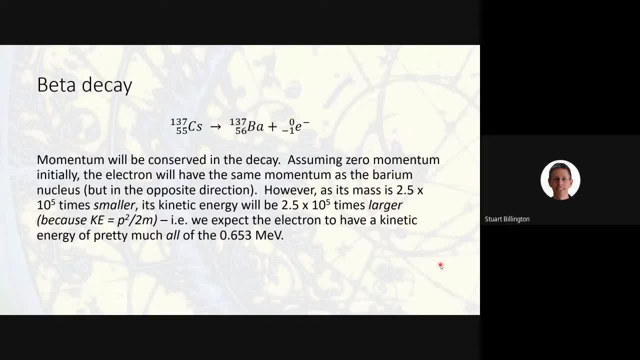 than the electron. so it's going to be 2.5 times 10 to the 5.. so if you remember that momentum is mass times velocity, and if the momentum has to be the same but the barium's mass is 2.5 times 10 to the 5 higher, you're going to have to acknowledge that its velocity is going to be 2.5. 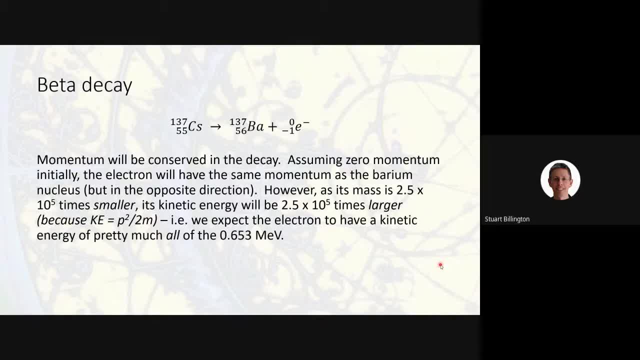 times 10 to the 5 smaller, so that the um, the two momenta, are equal for the barium and the electron x is going to be larger than it is with respect to the homogenous produc對 all of the 0.653 mega electron volts. the barium just gets so little velocity that basically it 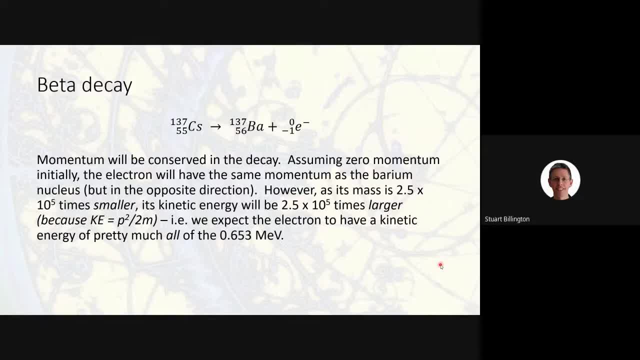 has very, very little kinetic energy. what this means as a prediction is that we expect all of the beta particles to come out of the cesium nucleus with the same kinetic energy and therefore the same velocity. and therefore, if we measure the kinetic energy of the electrons that are emitted, we expect to get a single figure of 0.653 mev every single time we do the measurement. 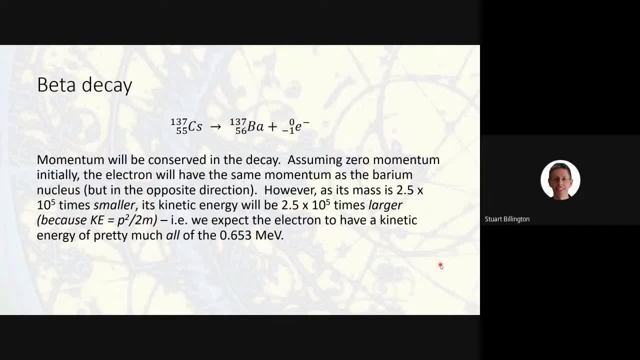 now to be clear before i put the next slide on um, if i'd have written an alpha decay equation up there and that had been an alpha part particle instead of an electron, and we'd have done exactly the same calculation and we'd have got a prediction of the energy, uh, and then we went away and measured the kinetic energy of the. 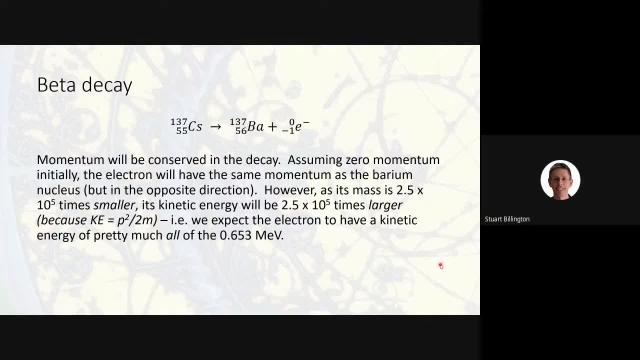 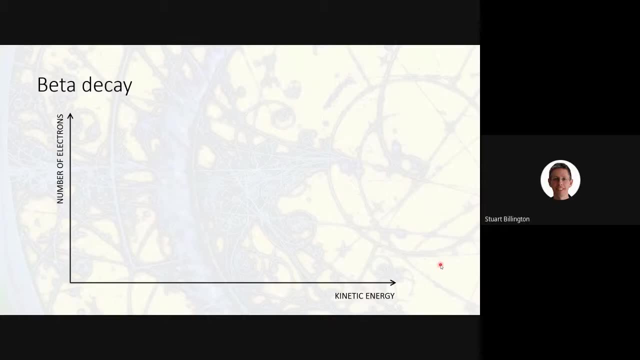 emitted alpha particles. uh, it's bang on. every time the prediction is perfect, but for the emission of the beta decay it isn't. uh, it's very, very wrong. so here's a graph of, um, what we do detect when we look at the beta particles that are emitted. so, uh, we'll do a frequency graph. so, across the bottom, 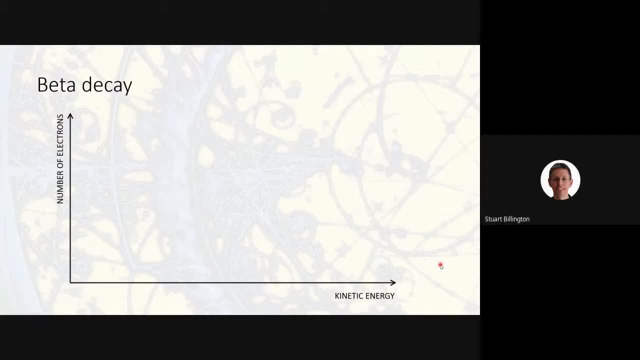 is kinetic energy, and up the side is the number of electrons that we detect with that energy. so we would expect just a spike up here somewhere. this is our prediction of 0.653 mev, and we would just expect all of the electrons to have this energy here. however, what we actually 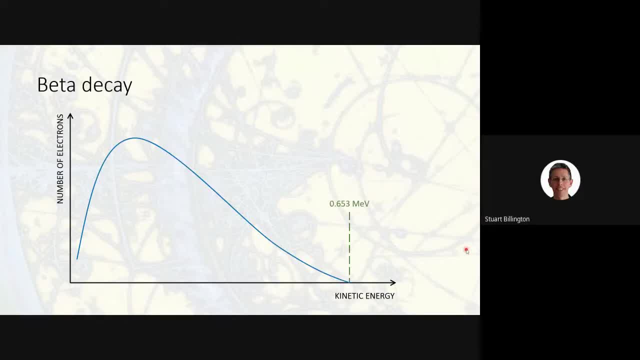 get is this shape of graph. it turns out that not a single emitted electron is ever observed to have 0.653 mev. not one, not ever. in actual fact, uh, the majority of the electrons uh have a kinetic energy far, far less than the predicted maximum. we do get some electrons with. 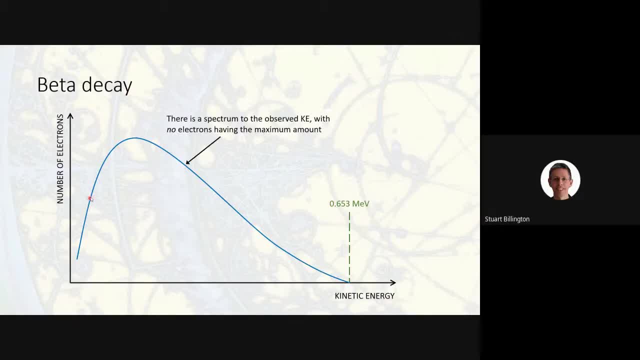 more kinetic energy and we do get some electrons with less kinetic energy. but it is definitely a spectrum rather than a single line, and the peak of that spectrum is nowhere near the predicted value. what this is an example of is a scientific theory making a prediction that, when tested, 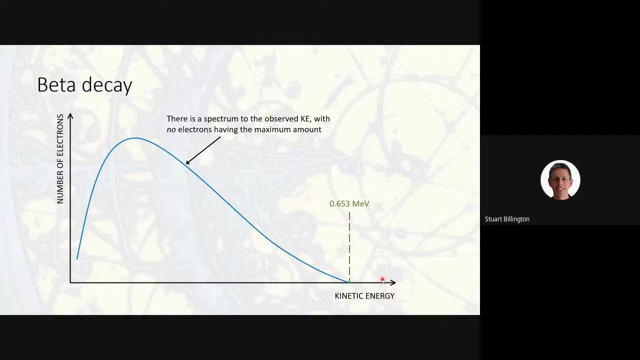 against experiment comes up, not just slightly off, but wrong, just plain and simple wrong, and what that means is that we have a theory that makes incorrect predictions and therefore our theory itself has to be considered as incorrect. we've done something wrong, we've made an incorrect assumption and we need to go back to the drawing board and fix it. 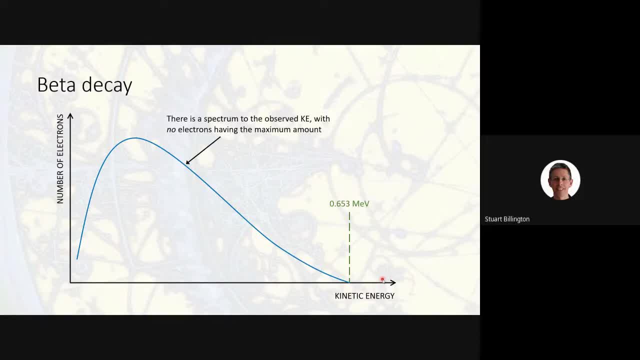 there is no amount of tweaking that is going to um fix this result. we've we've made a mistake, and the mistake we've made is by assuming that the beta particle was the only particle that came out um. what we're actually um seeing in this graph is that if this is the maximum amount of kinetic, 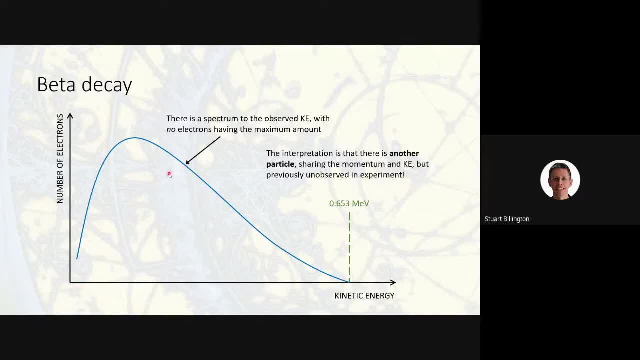 energy, then the beta particle only ever gets some of it. this beta particle here only got, say, half of the energy. where did the rest of it go? well, we must be missing a particle, there must be a number of particles missing a particle, there must be a number of particles missing a particle. 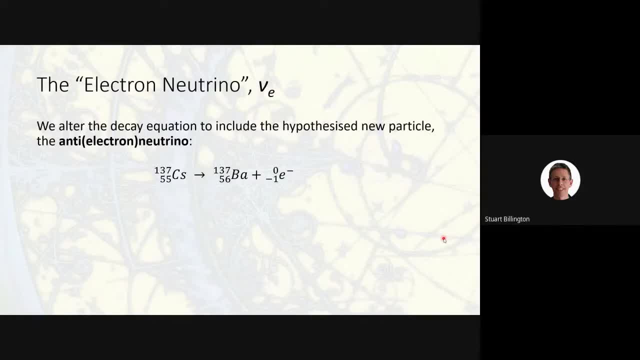 that's coming out. so this as the basis of our decay equation is an incorrect model and in actual fact, we need to hypothesize that there is another particle that comes out. this particle must be fairly shadowy, because if it was detectable easily, we'd have detected it. our detectors are very, very. 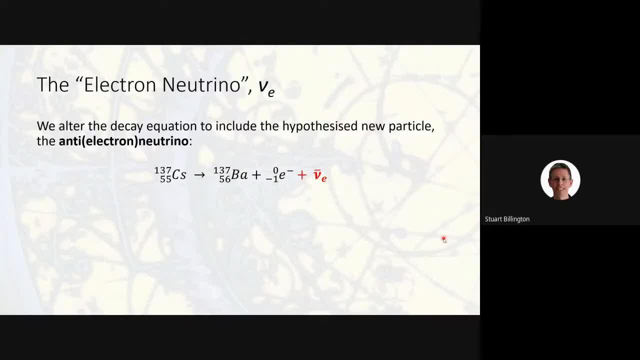 very good. and the fact that we don't find this, uh, this extra particle come flying out, means that it must have interesting properties that aren't like the beta particle, they're not like the electron. um, so a physicist, uh, an italian physicist called enrico fermi. 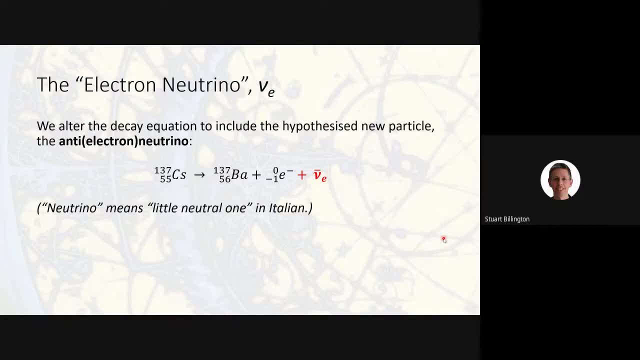 um, he gave it an italian name, which means little neutral one, the idea being that if it had very much mass, it would have collided with something and we would have noticed. and if it had any electric charge, it would have collided with something and we would have noticed. and if it had any electric charge? 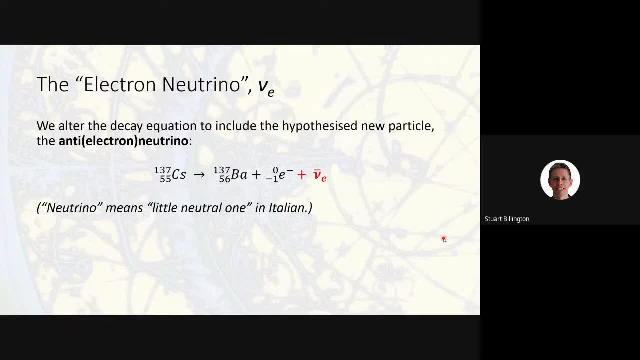 then it would have interacted with something electromagnetically and we'd have noticed. and so fermi is predicting that this particle has practically no mass and no electric charge. in actual fact- and i think i mentioned this in the previous lesson- um, in the standard model of nuclear physics, um, we treat the mass of the neutrino to be: 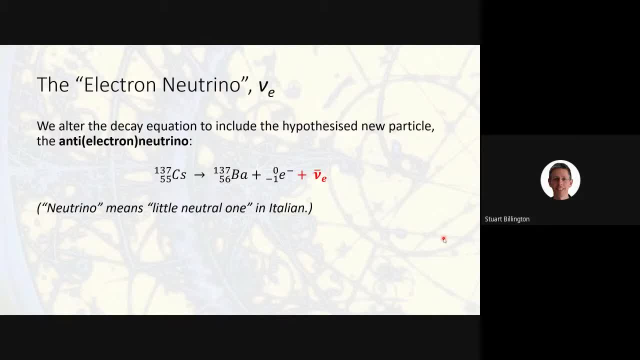 actually zero, a totally massless particle like the photon of light. in modern experiments the last decade or so we're fairly sure that the neutrino does have a very, very small amount of mass, but that hasn't been absorbed fully into the standard model yet because experiments are still ongoing. but whether it's zero or very, very small, it's practically zero. 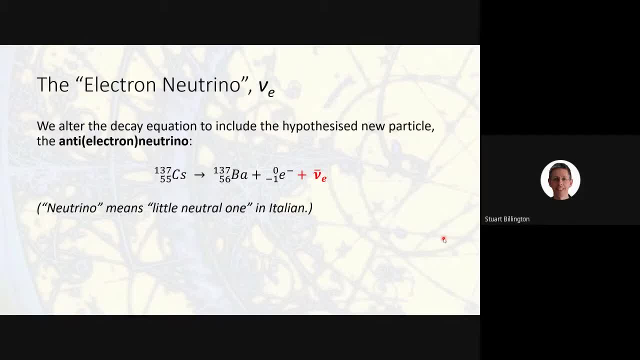 um for the experiments that we're talking about today. so the neutrino manages to escape from the elements falling right out of space and, yes, momentum is conserved. um, it never gets very much velocity and therefore it never gets very much kinetic energy. okay, so we now need to ask ourselves the question where? 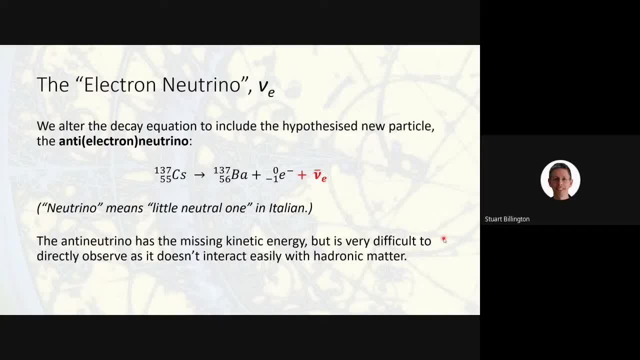 is it in our physics that predicts that a neutrino can be created? um, because if we can nail that down, we might be able to look at the properties of a neutrino, predict the properties of a neutrino and therefore we might be able to predict how it can be made to interact with matter. 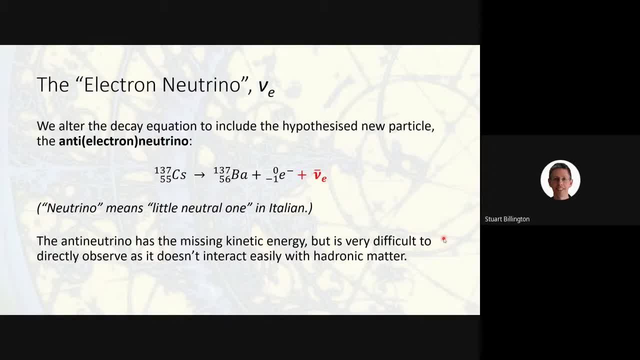 and therefore we might be able to create detectors that can detect it, to validate the model. so we need to ask ourselves the question: where is it in our physics that predicts that a neutrino can be? we need to go back to beta decay now and we need to ask the question: how is it that we could create? 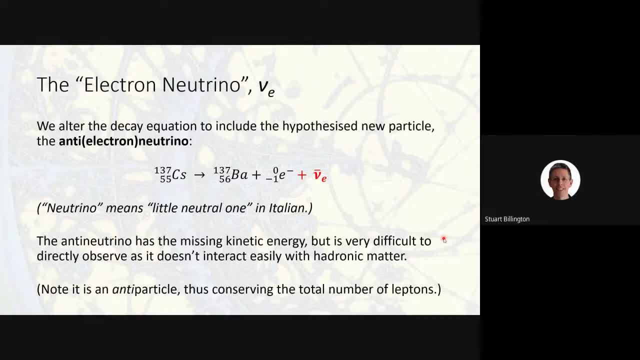 an extra particle. uh, just before we move on, just to note um, as the, as the model develops and as we understand more about the properties of the neutrino, um, we, we appreciate. you will appreciate in a few slides time that the neutrino is always produced alongside the electron and the two. 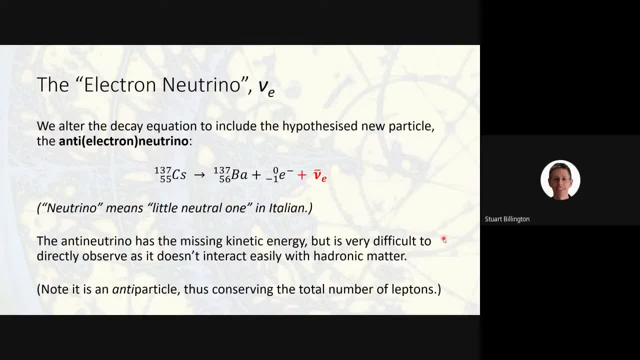 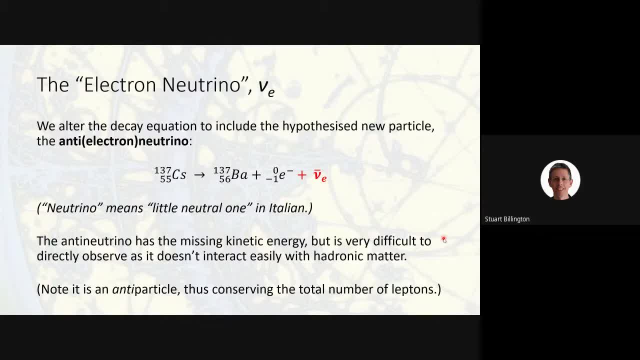 so if you create a lepton, you must create an anti-lepton with it, so that the total number of leptons in the universe doesn't change. as i told you when we were doing the particle models lessons. this might sound like we're just making up a lot of rules, but actually all we're doing is paying. 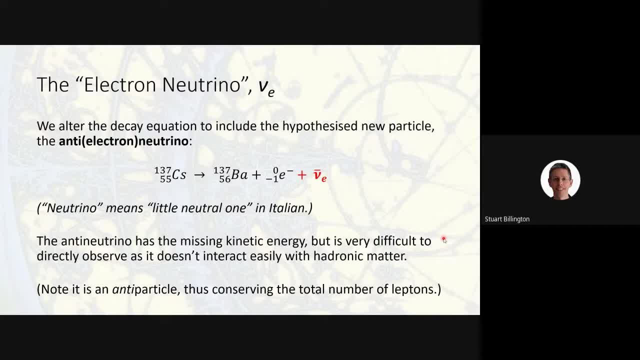 attention to the universe and writing down what we see to be happening and what we have never, ever seen in any experiments. since we did get good at detecting neutrinos, we have never seen any neutrinos be created without uh, their corresponding electron, or or muon or tau, and it's always an 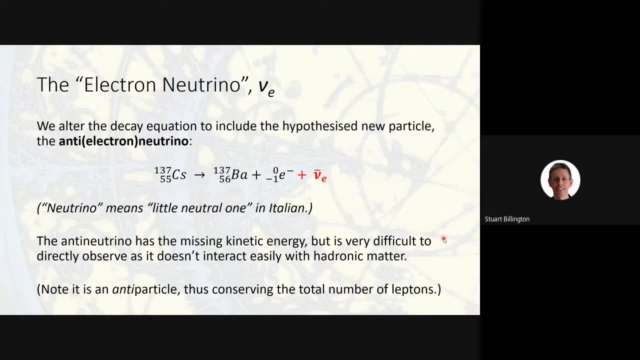 anti-electron neutrino with the electron- although to be honest, it is semantics, because you can call it an anti-neutrino or a neutrino, it's your new particle. you can call it what you like, but those are the rules. we always conserve the number of leptons. therefore, if you've got an electron being produced, 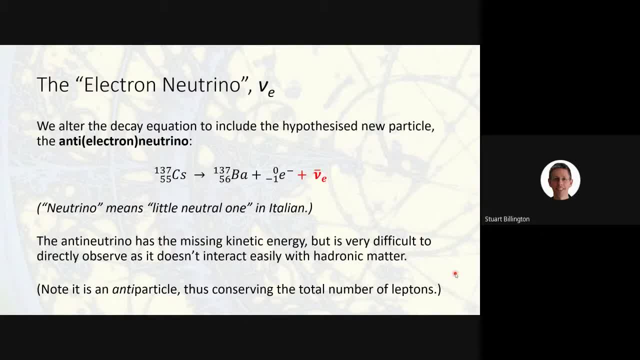 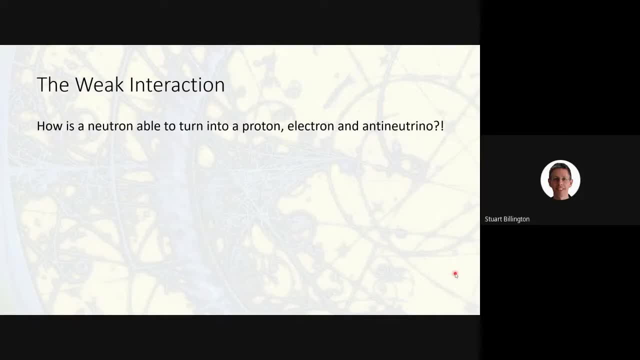 you need an anti-electron neutrino to go with it. okay, so where did the neutrino come from? and, in actual fact, while we're at it, how did a neutron manage to turn into a proton and an electron in the first place? anyway, we glossed over it at gcse. if i taught you at gcse, i said something like: 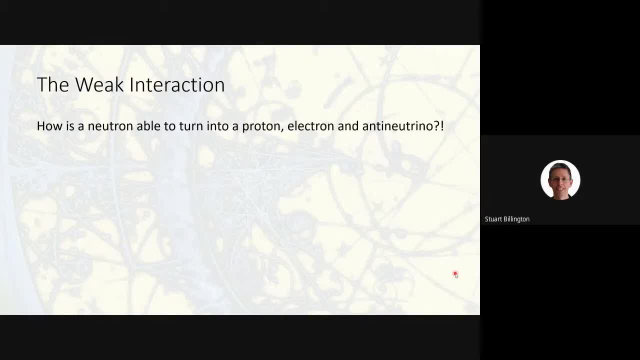 the, the neutron ceased to exist and, in its place, a proton and an electron uh began existing. but that was just hand waving, and if we want to do this properly at a level, we need to ask: what is the mechanism, what is the? what is the process by which a neutron turned itself into a proton and 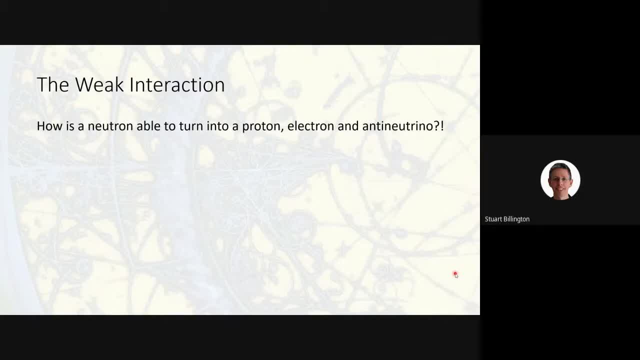 an electron, and now we find an anti-neutrino as well. uh, maybe we can't do that now, so we're just going to try it again once we've tried it and we try to explain what happened, and maybe this will give us some idea of the properties of the anti-neutrino and allow us to detect it. 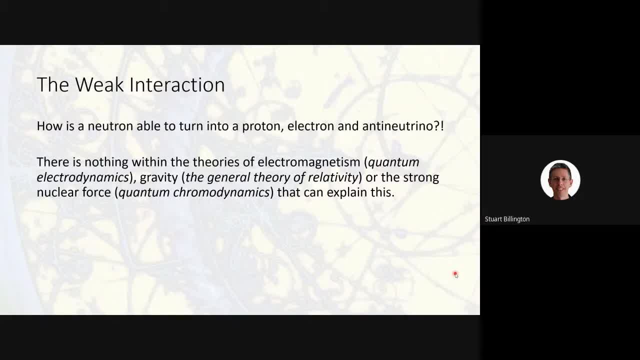 okay. so we uh spent a long time in the 1970s having a good look at the existing theories of electromagnetism and gravity and strong nuclear force and it turns out that there is no aspect of any of the three known forces that can cause a neutron to turn into a proton. there's nothing. 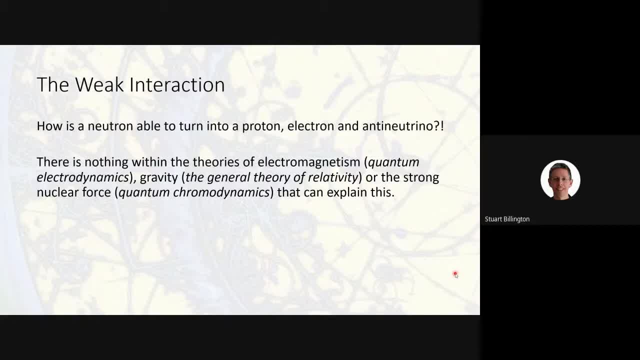 the equations, any of the principles of the models. there's just nothing there, and therefore we have to conclude that we are discovering some brand new physics that we need to add to the standard model, or what became the standard model, to account for beta decay. so it's not often that a single isolated 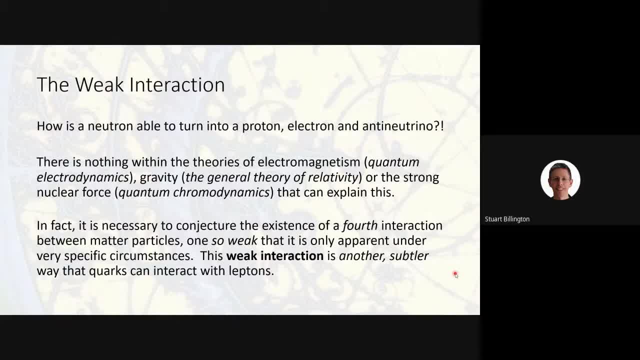 event, beta decay. it's not often that a single thing causes us to invent a whole new area of physics, but that what- that's what beta decay has done for us. we have to turn our attention to a whole quarter of physics that we've been ignoring up till now. if we want to explain beta decay how. 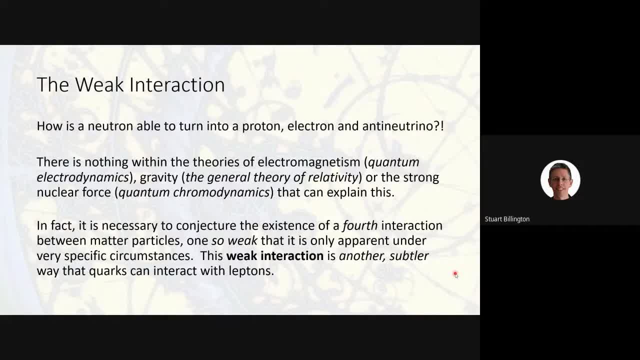 does a neutron turn into a proton, an electron and an anti-neutrino? so all we can say for sure is that if this fourth force, this fourth interaction of matter particles had been in any way strong or noticeable, we would have seen it in other situations by now. 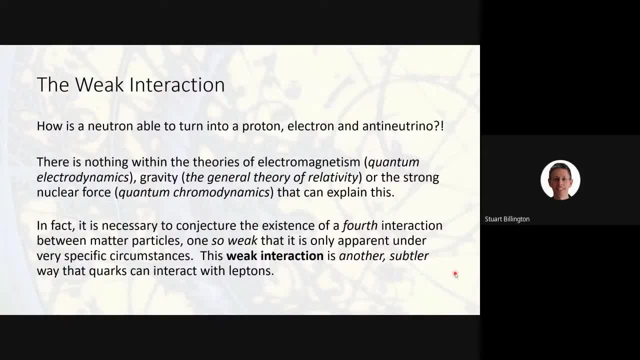 so, like we said that this strong nuclear force must be very, very strong to be able to overcome the coulomb force, what we can say about this new fourth force is that it must be very, very, very weak, because basically it should be very, very weak. doesn't appear to do anything except beta decay. 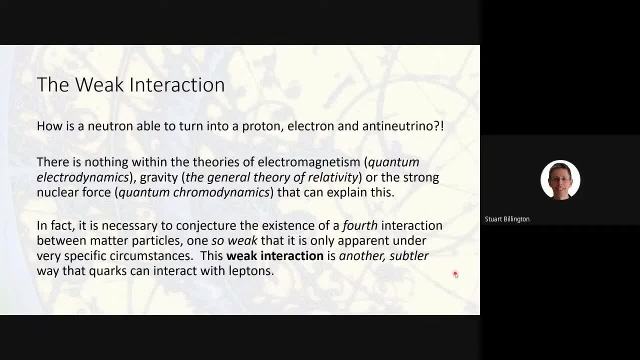 Likewise with the strong nuclear force. we said it was a strong nuclear force because if it exerted itself outside of the nucleus, we denoticed. Well, same thing with this weak interaction. It must be a nuclear force, otherwise we denoticed it. 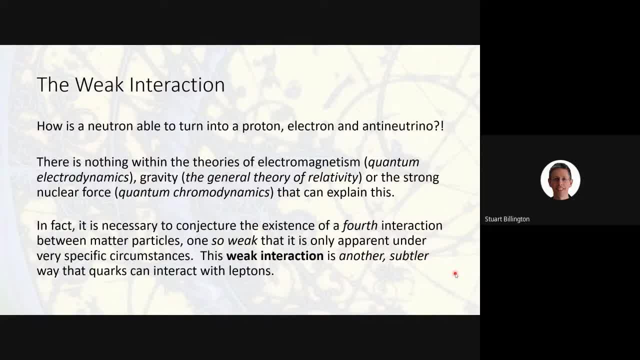 So it's up to you whether you call it the weak nuclear force in mirroring the strong nuclear force, But these days it tends to be called the weak interaction, And what it is is a process that quarks undergo at a deep down, fundamental level. 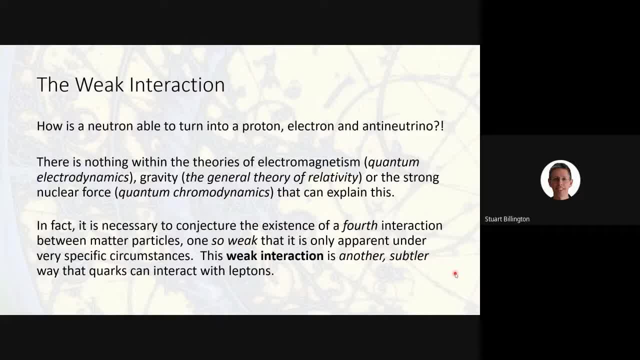 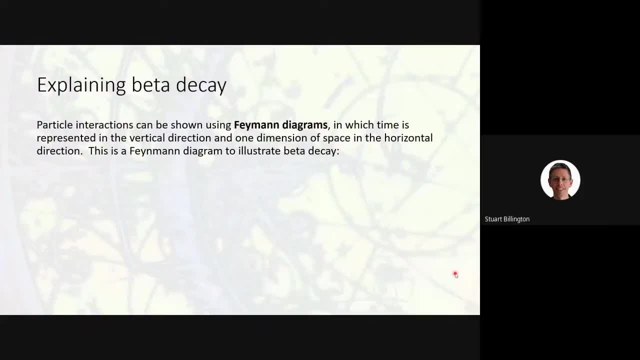 either with themselves or with leptons. So let's have a little look at what the weak interaction is. OK, so I'm going to show it to you diagrammatically, using the tool that Feynman invented. Just to be clear from the outset. 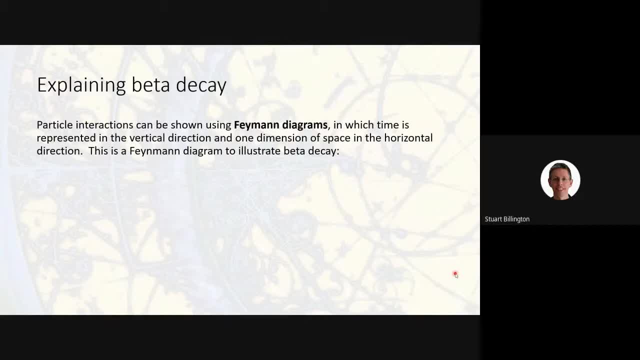 you will not be examined on these Feynman diagrams. They're not on your specification and they will not appear on your exam. You do not need to revise them, You do not need to be able to draw them, You don't even need to be able to interpret them. 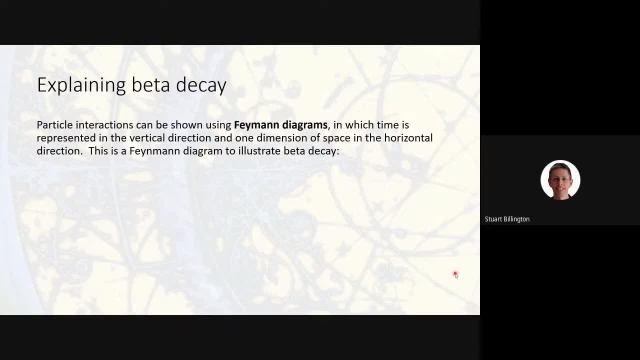 However, they are an incredibly powerful visual tool and there is no simpler way of explaining beta decay other than by these diagrams. So I'm going to show you the diagram, OK, But you don't need to be able to reproduce it, OK? so in a Feynman diagram up the page is the time axis. 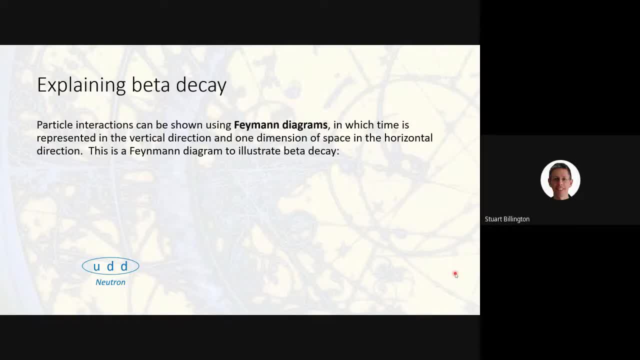 So at the moment I've got the neutron down kind of now at the bottom of the page And in the space that is above the neutron, that's the neutron's future. So over here we'll have what's happening next to the neutron. 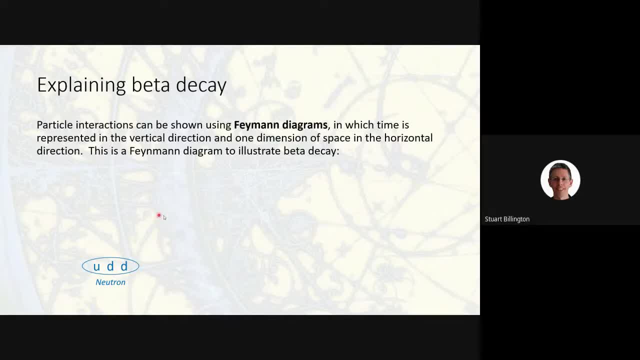 Left and right. We'll take it to be left and right because it's left and right on the page. It's just a one-dimensional time axis across the page. So let's have a little look at what happens to the neutron. So inside the neutron, the up quark and the down quark. 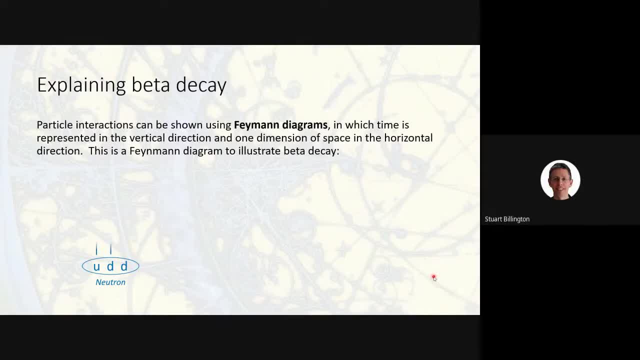 they don't do anything at all, They just sit there. They haven't moved left and right, which means that they haven't moved the neutron in the right direction. So they're not moving left and right, They're just sitting there. They're not moving left and right, which means that they 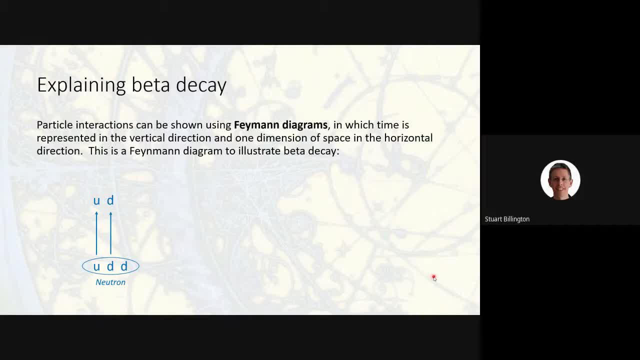 haven't moved in space, And all they've done is continue their existence into the future. So this was then, This is now, And the up quark has done nothing at all. It's just continued to sit there in the same place. 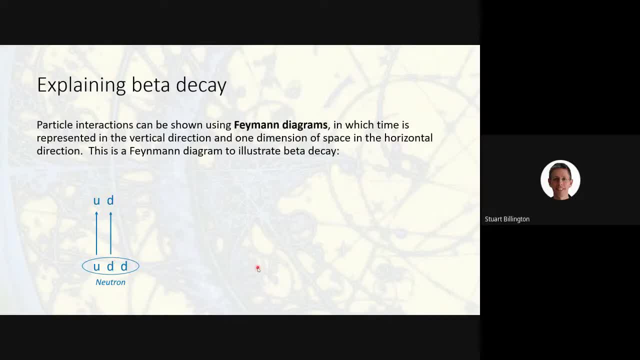 And the down quark has done nothing at all. It's just continued to sit there in the same place. If the other down quark had continued to do exactly the same thing, we now have a problem Because at some point during its journey into the future, 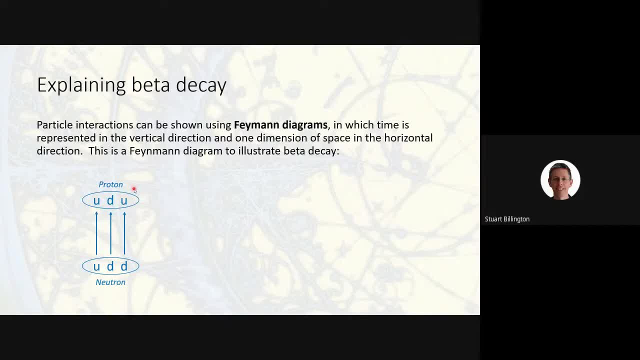 the down quark just turned into an up quark And that's where I left it with you at GCSE, with no explanation other than it just happens. But now at A-level, that arrow isn't good enough And we need to get rid of that. 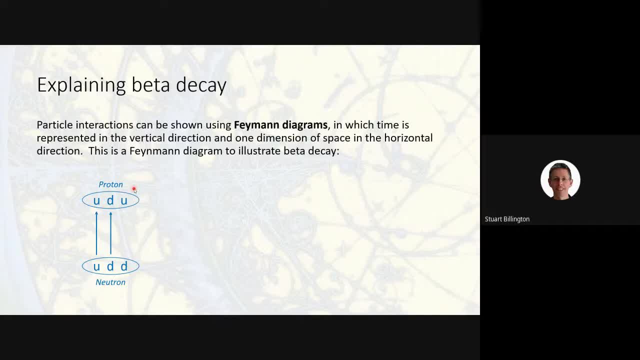 And we need to replace it by what really does happen. So what do we think happened? Well, in the weak interaction, we think that the down quark decayed, And that's a good thing, And that's a good thing. We think that the down quark is a heavy particle. 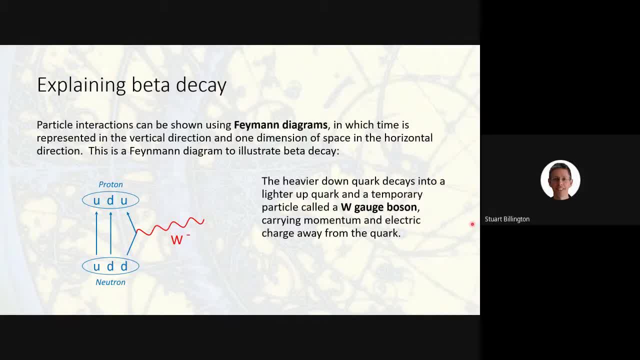 It has more mass than it needs to have And that, therefore, in a quantum, mechanical, statistical universe in which randomness is at play, we think that it is likely that, in enough time, the down quark will realize, or the universe will realize, that 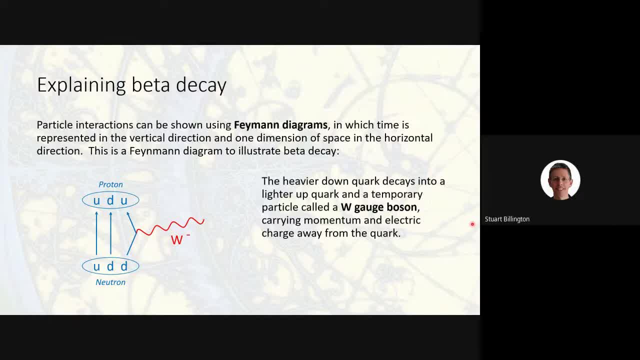 energy can be minimized further by the down quark shedding some mass, And so what we think happens is that at some point the down quark emits a little bit of its mass, turning into a lighter particle, And we recognize what the lighter particle is. 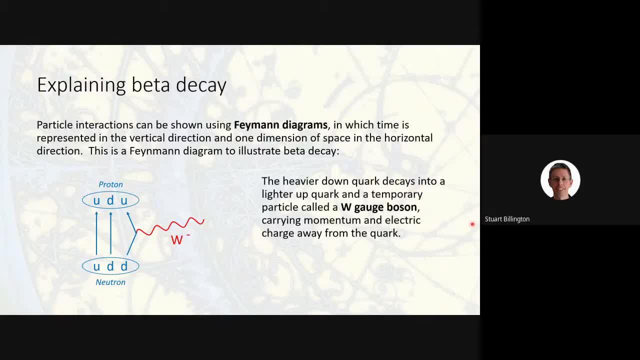 It's our friend the up quark. So we think that what happened inside the neutron was that the down quark was jostling around just a little bit. It pulled itself slightly to the side, emitted a little piece of itself by decaying. 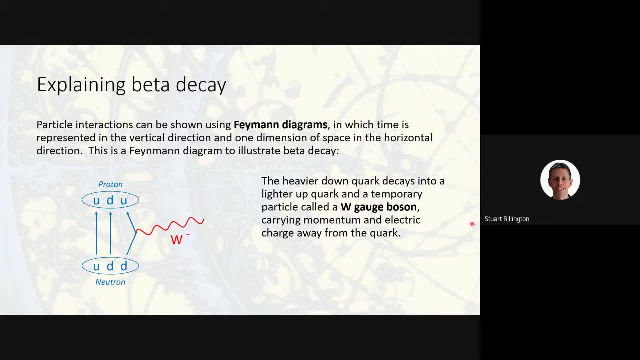 into a pair of new particles. One of the particles was a quark and remained bound by the strong nuclear force to the other up and down quark. So when the down quark decayed and became an up quark, the up quark was bound and couldn't leave. 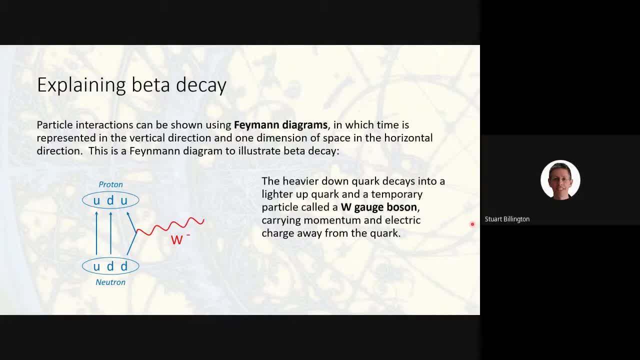 And that's why the neutron became a proton. However, a little piece of matter managed to escape And we've needed to give a name to this little piece of matter, So we gave it a really great name. Started badly by just calling it a letter of the alphabet. 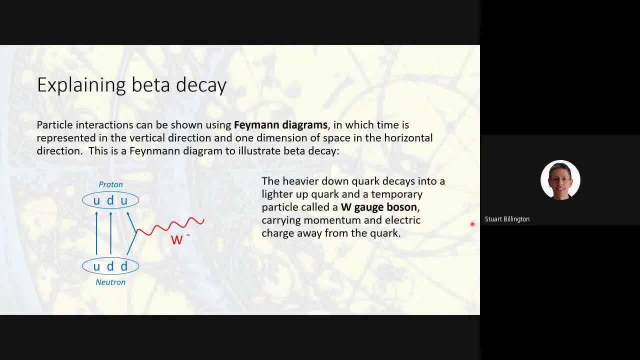 but then followed up with gusto with gauge boson. So it's the W gauge boson. OK, What does that mean? Well, first of all, it's not examinable, so don't worry about it. But bosons are particles that don't have to convey. 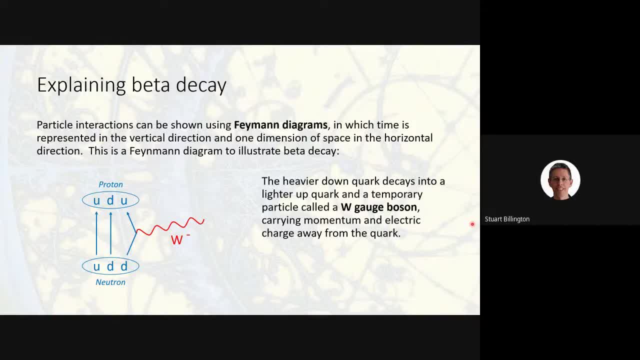 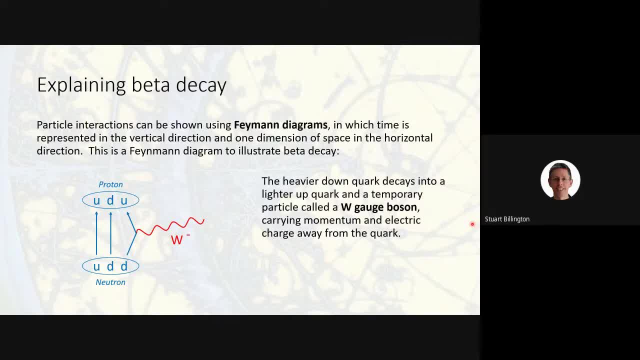 We have to conserve energy, but we don't have to count the number of photons. There's no rule in the standard model of nuclear physics that photons must be conserved. There are rules about conservation of quarks and leptons, but not photons. 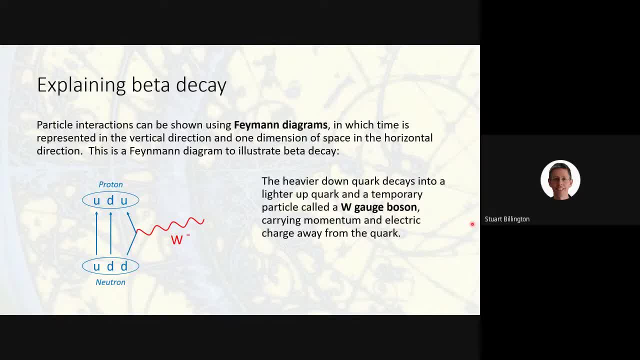 And the W is in the same category as the photon. It doesn't need to be conserved. It can be created and it can be destroyed at will. Its properties can't So any momentum or energy or, in the case of this, W. 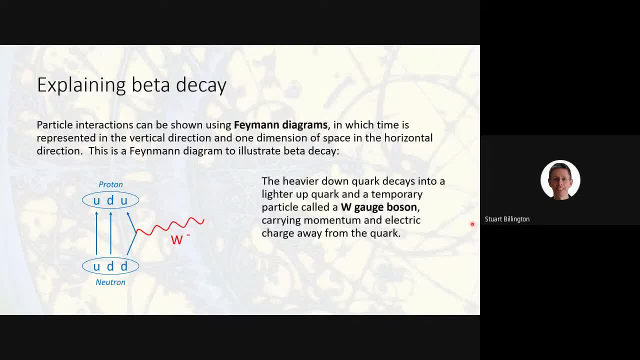 particle charge. its properties must be conserved, but the particle itself doesn't have to be, And very, very, very loosely, that's what we mean by the word boson. It doesn't mean it's not a conserved particle. 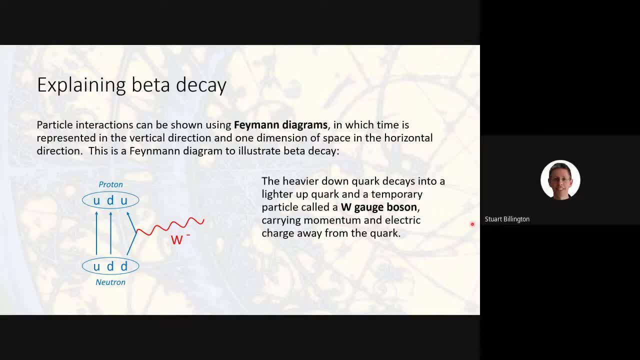 It's a temporary particle. It exists fleetingly. So the down quark has decayed into a permanent up quark, which has remained bound in the nucleus, and a temporary fleeting boson that isn't going to last very long at all. 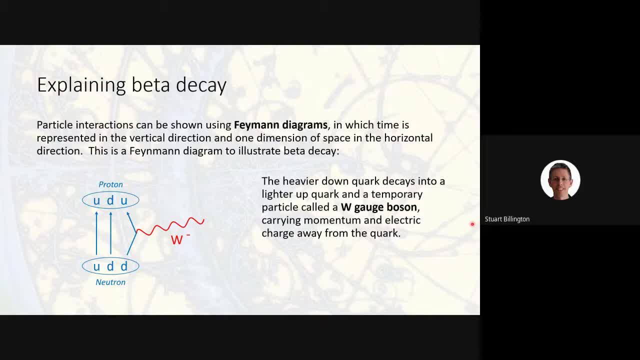 The physics of the bosons is part of the standard model, but it's not part of your A-level. So if you want to know why the W doesn't exist for very long, well, take a degree in physics And by about your third year you'll. 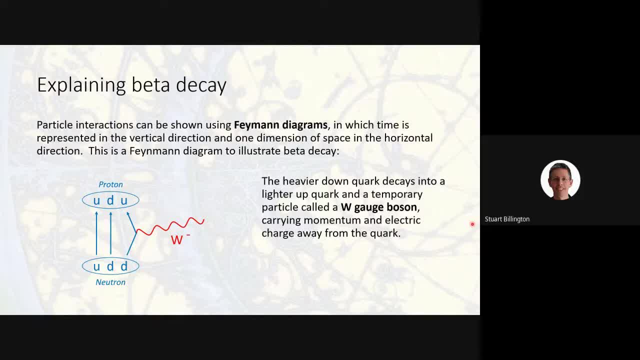 do some particle physics that is at a high enough level that you'll get your head around that a little bit. So notice that it's a W minus. It's a charged particle because the down quark had some charge and the up quark has some charge. 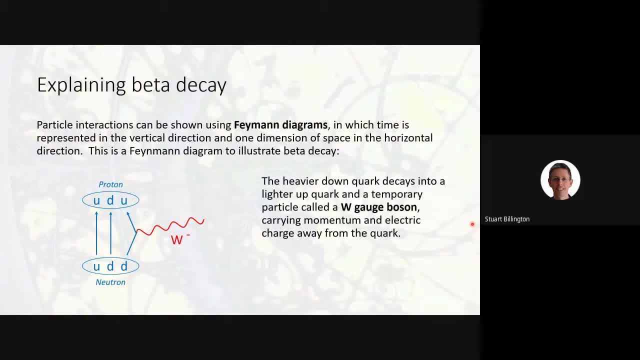 But there's a difference. The down quark is 2 thirds negative, The up quark is 1 third positive. So the down quark has lost all of its 2 thirds negative and then it lost another third of negative to leave a particle that. 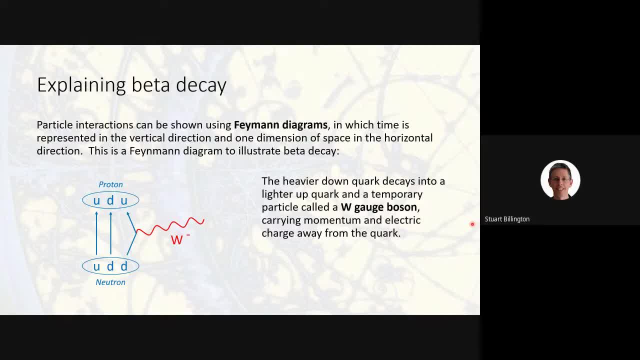 was 1 third positive, 1 third A, So altogether the down quark lost an entire 1E lot of charge and that's why it's a W minus. So the W is carrying a little bit of momentum, a little bit. 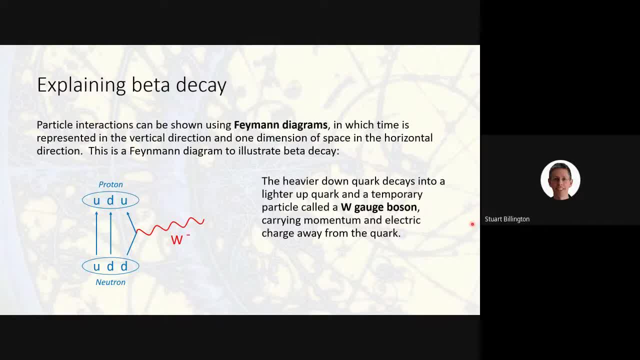 of energy and a little bit of mass and a little bit of charge. The W is not going to exist for very long, but those properties must continue to. So the W decays Again. same principle: It's got mass and energy and it's more stable. 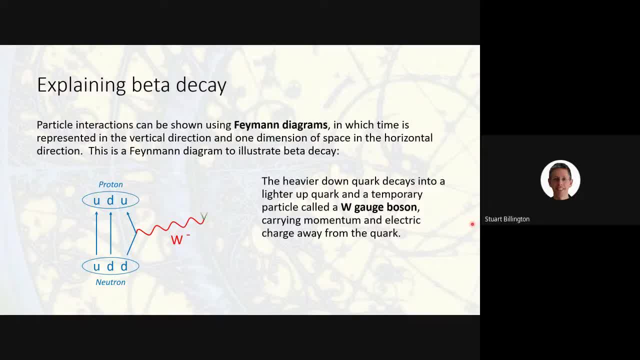 It's going to be stable as lighter particles, So the W is going to decay into our friends the electron and the anti-electron neutrino. The electron carries away the mass and the negative charge and between them they share the kinetic energy. 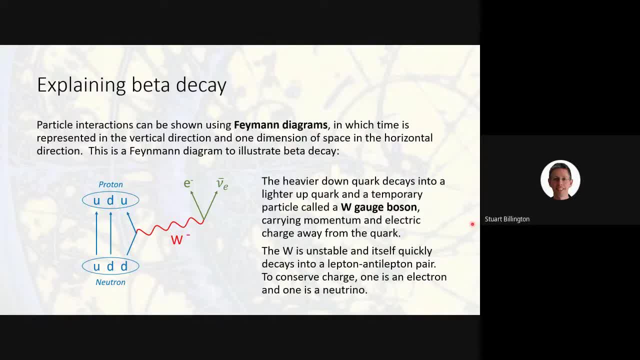 One more time: the W minus is not examinable on your A level. But you shouldn't have an A level in physics if you've never been exposed to these ideas. But in terms of what's examinable, it's just the beginning bit and the end bit. 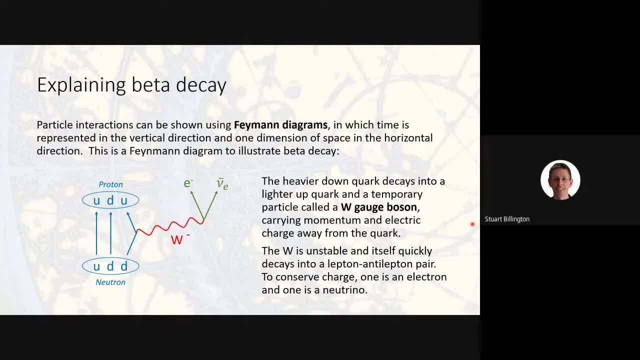 The process in the middle is not something that you're going to need to be able to reproduce in an exam. It's just there because I think you should know it. OK, so that's your Feynman diagram. This presentation is on Google Classroom. 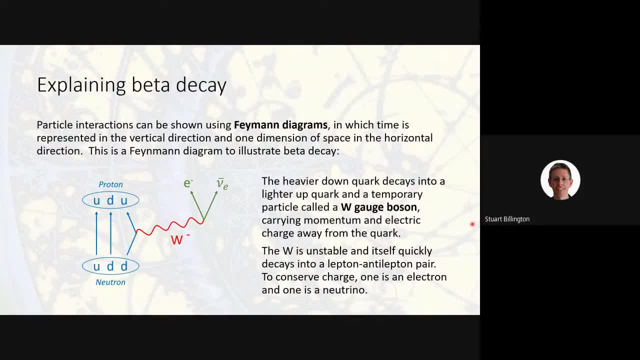 I suggest you play the simulation a couple of times to see the process happening, just to make sure you're happy with it And just before we leave the diagram behind. just to be clear, the red wiggly line is a symbol that represents the W I. 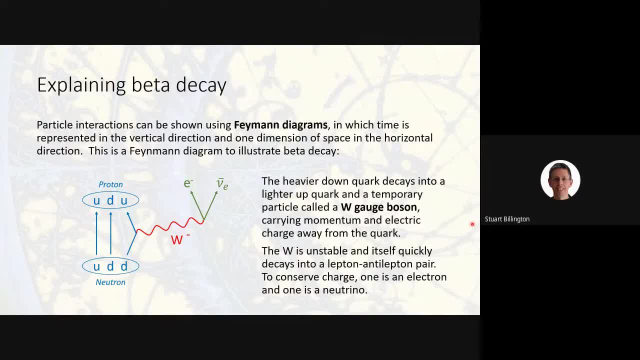 don't want you to take the wiggly line literally as the W snaking its way through space. OK, That's not what's happening there. The W travels in a straight line, just like all particles. It's just that we use a symbol of a wiggly line. 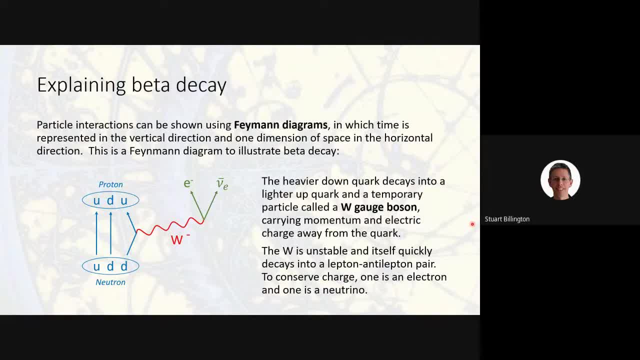 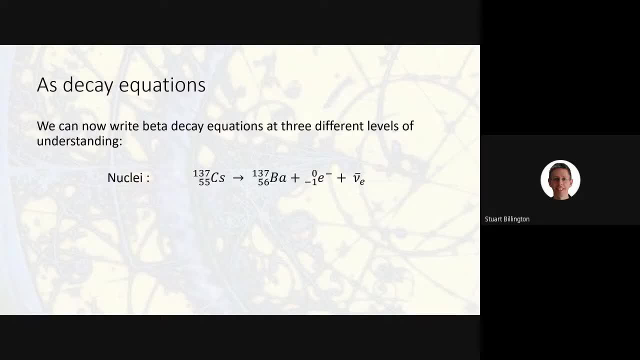 to represent it. OK, so the bit that you do need to be able to reproduce are some equations like chemical equations. You've seen these before. We've seen some today, So there are three different levels that we need you to be able to explain. beta decay at. 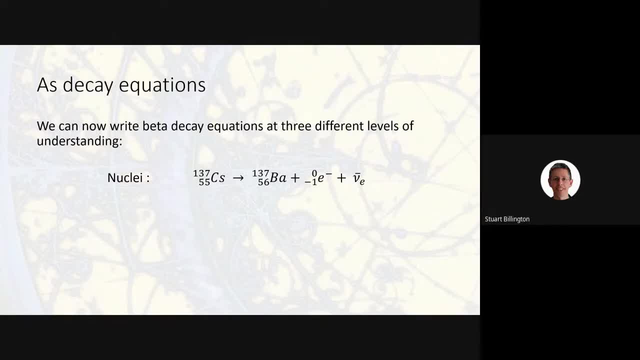 And when asked this question, I would say OK, well, what's the answer? And if you're asked in an exam question to explain beta decay, you need to read the question very, very carefully and look at the language that the examiner is using. 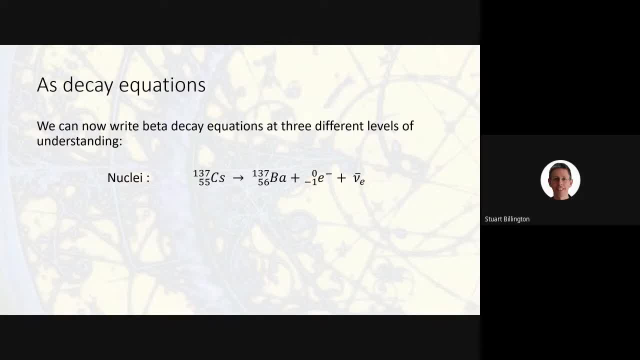 If the examiner is talking about nuclei and isotopes and elements and cesium and barium, then you are expected to give us a nuclear explanation of beta decay. So that's what's on your screen now: a nuclear equation. This equation starts with the nucleus of the cesium-137. 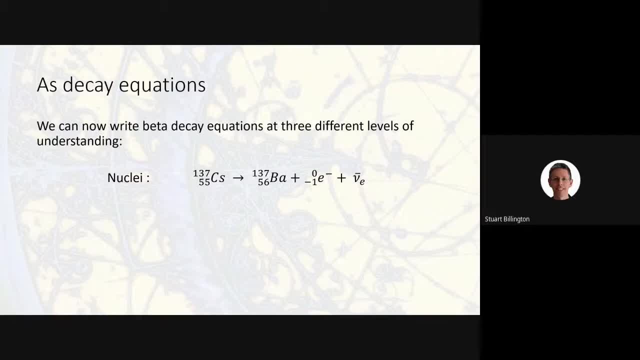 decaying into a nucleus of barium-137 and showing us the electron and the anti-electron neutrinos? Or the exam question might be talking about protons and neutrons, in which case we need an explanation in terms of nucleons, please. 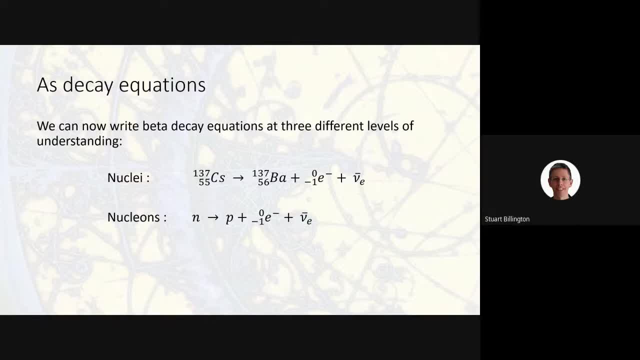 So could you please write an equation in which a neutron, an electron, transforms into a proton and the electron and the anti-electron neutrino, Or the question might be talking about quarks, And if the question is using the word quark and up and down, 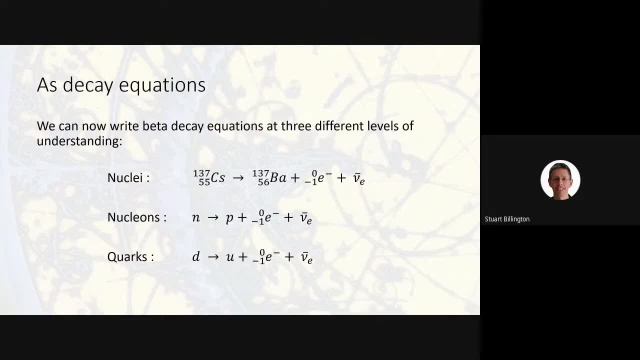 then we need a decay equation that offers an explanation in terms of the quarks, So a down quark decays into an up quark, and the electron and the anti-electron neutrino. So the right question is: what's the answer? 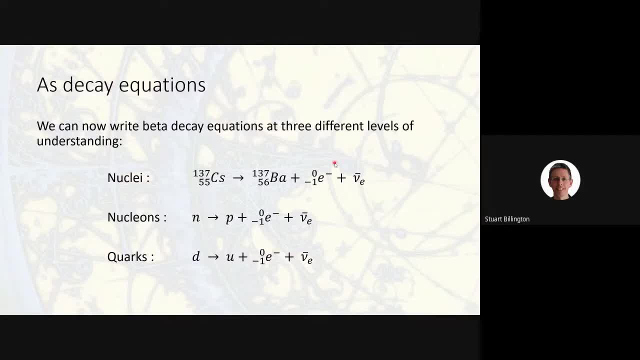 And the far right side, the electron and the anti-electron neutrino. it's always the same, It's just. are you telling me what's happening to the nuclei, the nucleons or the individual quark, And when you are talking about the quarks? 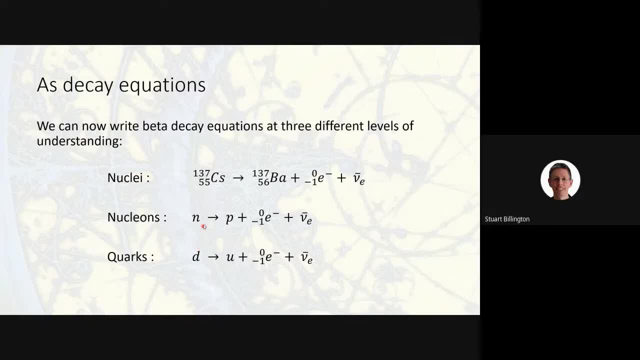 I only want to know about the quark that changed. So inside this neutron, remember, there is an up and another down that don't do anything, that just end up inside the proton. I don't want to know about those. I just want to know about the down that changed into an up. 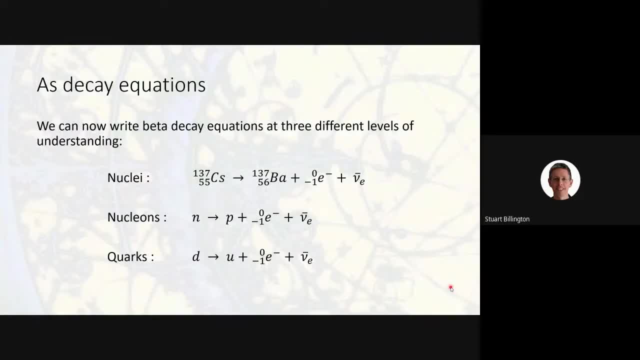 And what's happening now is that the down part is changing And there's been a couple of studies that are showing that's not happening And that's the goal of using the beta decay equation And, as you can see, that's the goal of using the beta decay. 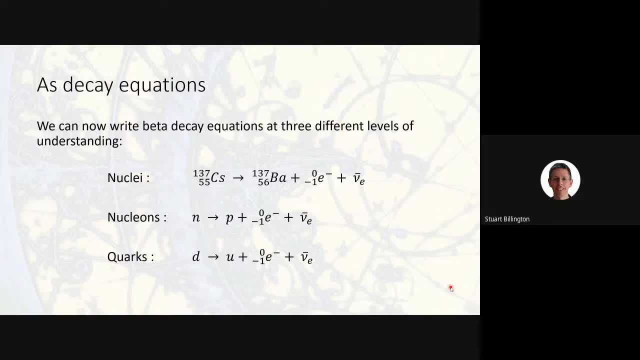 equation. So we're obviously going to lost the book, but we can make it change. So that's the goal And we have to look at some further questions. Now. we have got some comments about the silicon question, about the beta decay. 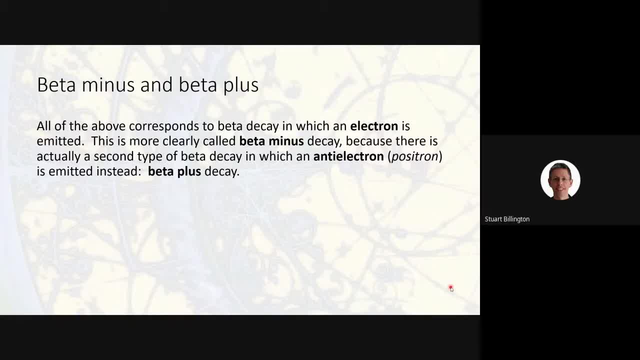 And it looks like there's the second question and I'm not sure if you've seen it. I'm sorry, I've got a question. Yeah, I've got a question. When you look at beta decay really clearly, it turns out that there are two types of beta decay. 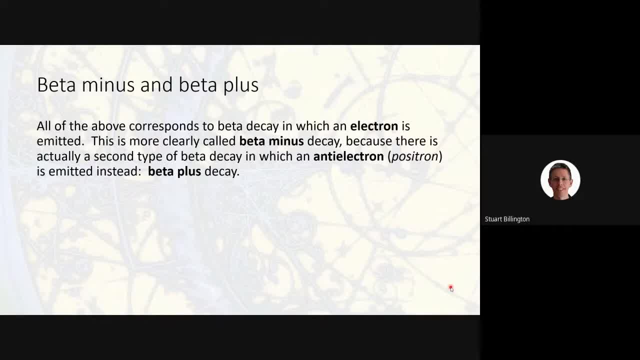 because there are two types of electron. There's the electron and the anti-electron, the positron- And it turns out both can be products from beta decay, And so when an electron is emitted, we need to start referring to it as beta minus decay, the minus referring to the. 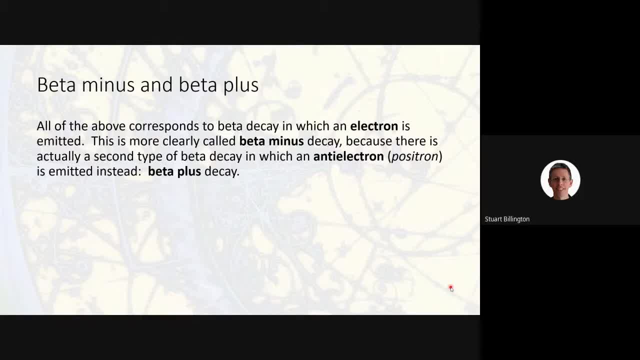 charge on the emitted particle. So when a negative electron is emitted, we refer to it as beta minus decay. But new for A-level is the existence of beta plus decay, in which the same process occurs, but this time a positron is emitted rather than an electron. 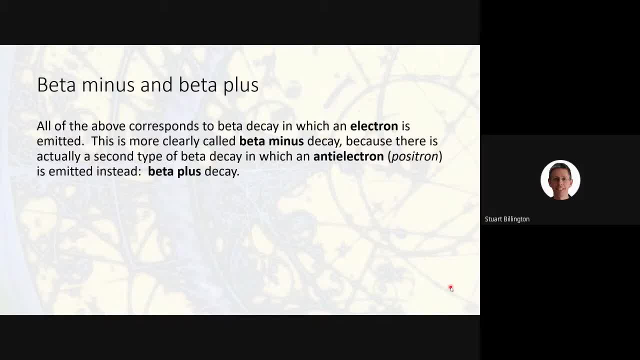 And, as a result, we get a negative electron And, as a result, we get a anti-electron instead of an electron. Okay, so one for you now. You've just written down the equations from the last slide. I hope I'll leave them on the screen for you in a second so that you can try to mirror them. 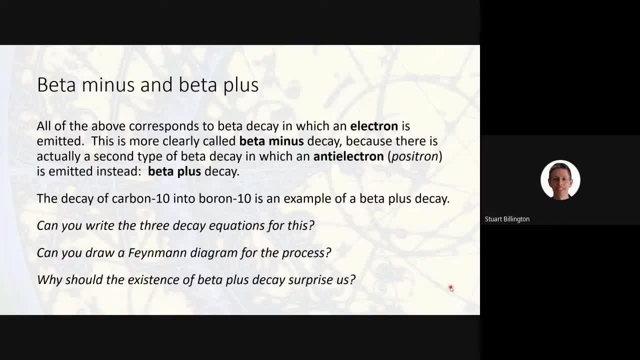 This is a different example now, So carbon-10 decays into boron-10.. And this is a different example now, So carbon-10 decays into boron-10.. As an example of beta plus decay. So what I would like you to do for me, please. 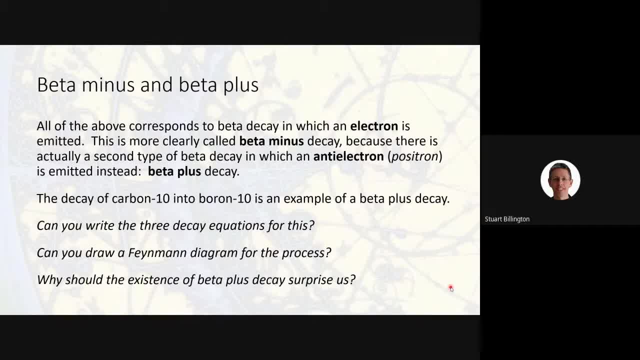 is, as a minimum, can you write down the three examinable equations for the nucleus, the nucleons and the quarks for carbon-10, beta plus decaying into boron-10? And if you whiz through that, you could have a go at drawing a Feynman diagram for it And in the back of your mind. 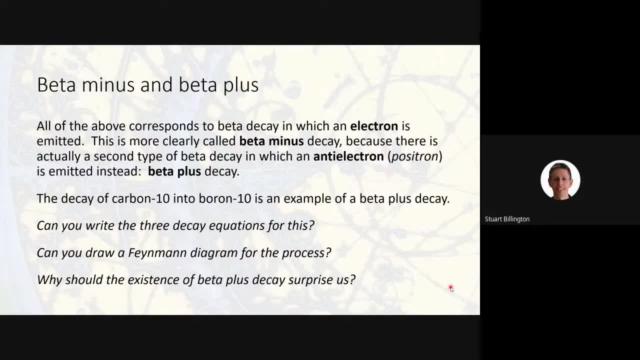 you need to ask yourself: why do we teach you about beta minus at GCSE but not beta plus? What is it that beta plus has that beta minus doesn't? that makes beta plus a surprising event. So I'm going to put the last slide on. 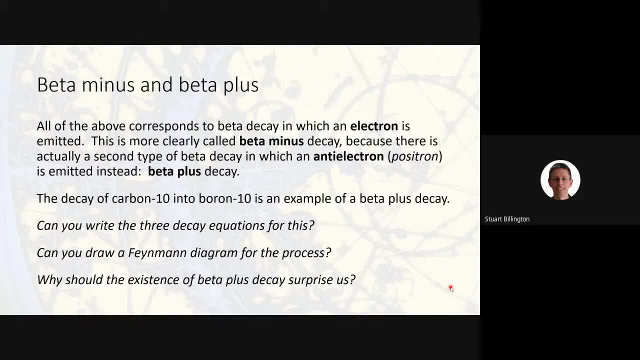 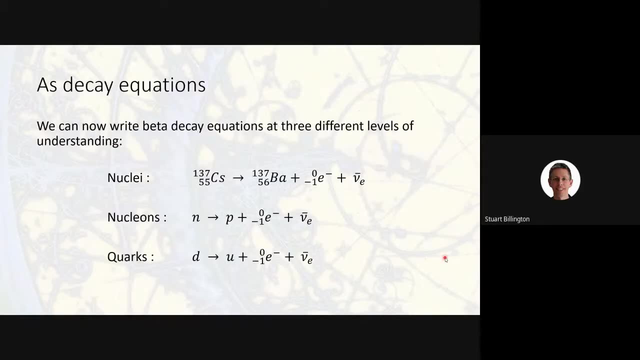 So that you can try to modify the equations of beta minus decay to produce the beta plus decay equations. But you won't be able to see this slide which says carbon-10 turning into boron-10.. Here's the previous slide. This needs to be carbon-10.. 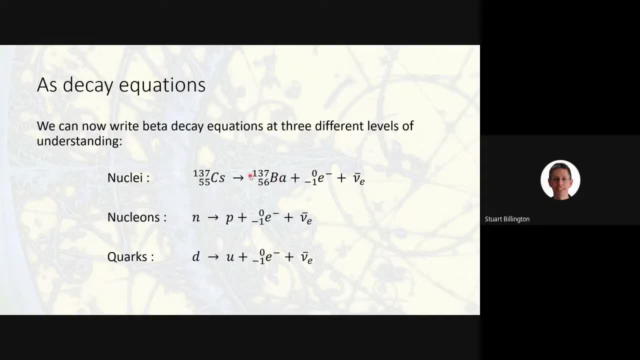 And this needs to be boron-10.. And carbon is element six. Okay, so carbon-10 to boron-10.. I'm going to give you three minutes. see if you can get the equations done, at the very least. 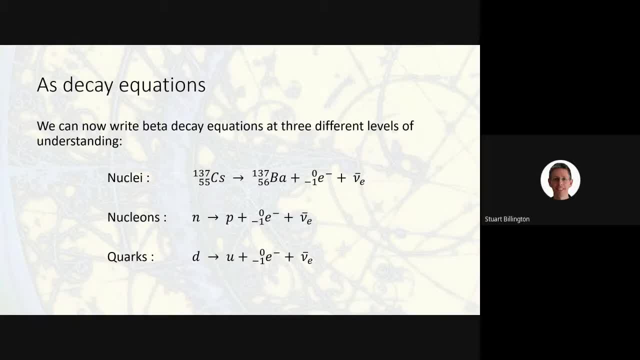 Okay, So you should have found that a bit tricky actually, So we'll see how you did. Okay, So here we go. There's your carbon, which is element six. 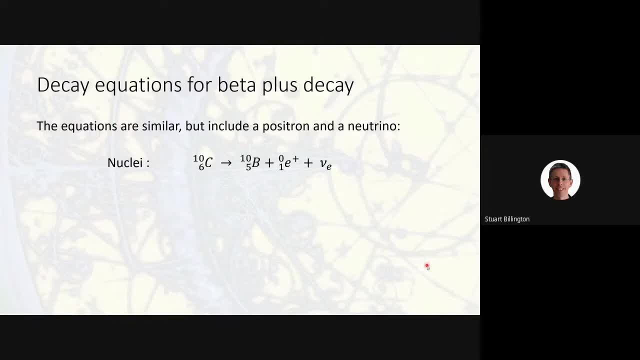 Boron's before carbon. on the periodic table, which some of you might have known, Boron's actually element five. But even if you didn't know that, you did know that a positron is being emitted, which means that an amount of positive charge. 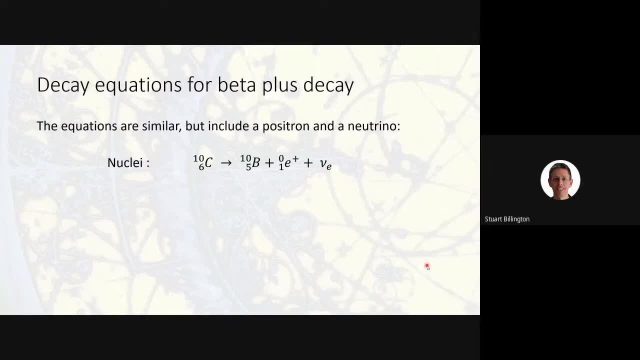 has left the carbon nucleus And therefore you should have been able to get a guess that if an amount of positive charge has left the nucleus, then it must have been a proton that ceased to exist inside the nucleus. So that's your decay equation for the nuclei. 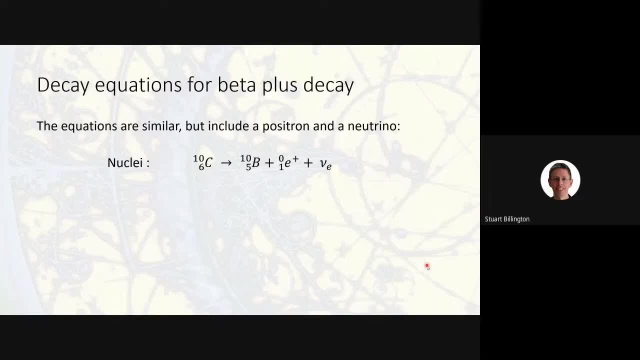 Notice that the neutrino no longer has a little hat on it For the previous equations here we put the little bar on the top of the neutrino to indicate that it's an anti-neutrino. So now no bar, and that indicates that it's just a fully-fledged neutrino. 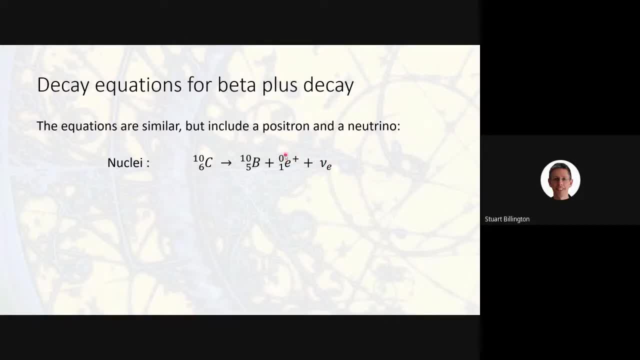 You might object to the fact that the anti-electron really ought to have a bar on top of it, but traditionally we never write a bar on top of the electron. Instead, the symbol for the positron is E plus, and that stems back from the fact. 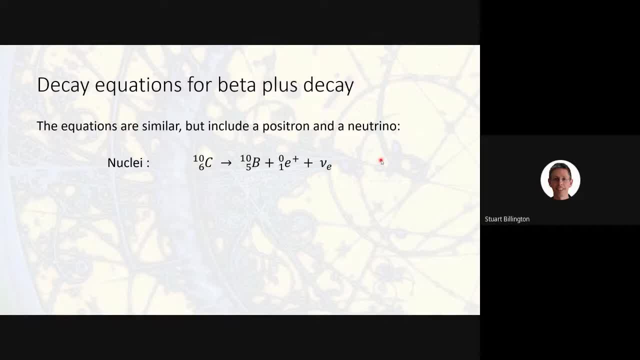 that Anderson discovered it before he knew what he was looking at, and therefore it got itself a name: the positron, and its own symbol. Okay, so we now need a nucleon equation And, as we've just seen, there were six protons. 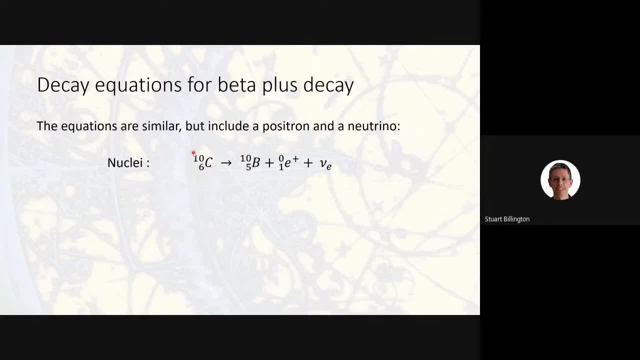 but now there are five protons, but the mass number hasn't changed, which means the number of nucleons hasn't changed. Therefore we've lost a proton, so we must have gained a neutron, And so that's our nucleon equation. 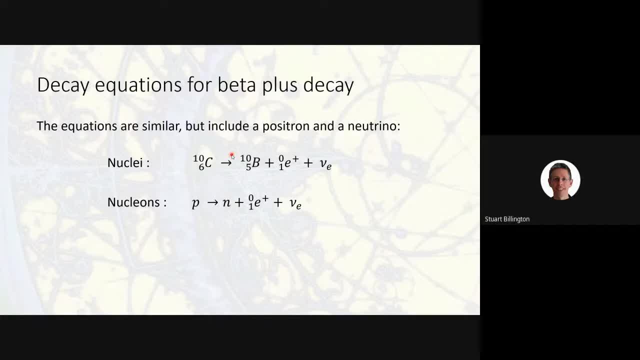 This time, instead of a neutron decaying into a proton, we have a proton decaying into a neutron, And again, charge is conserved. One lot of charge here, one lot of charge here. And leptons have been conserved. 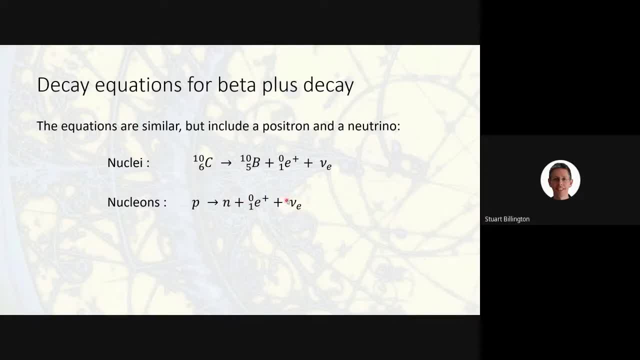 This is an anti-lepton, This is a lepton. So the total number of leptons in the universe is still zero. Well, maybe not the whole universe, but this equation. And then, at a quark level, a proton is two ups and a down. 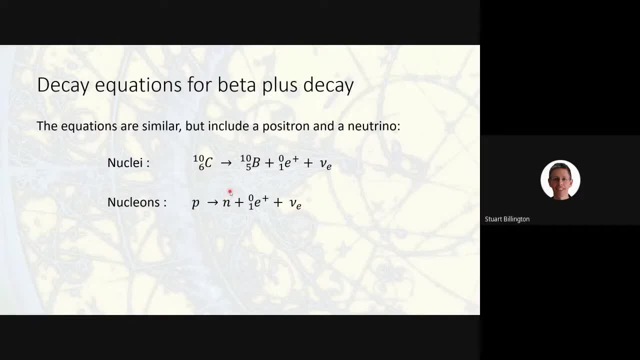 And a neutron is one up and two downs, And therefore one of the ups has turned into a down And that gives us our quark equation, So very, very, very similar to the previous equations. All we've done is swap the proton and the neutron round. 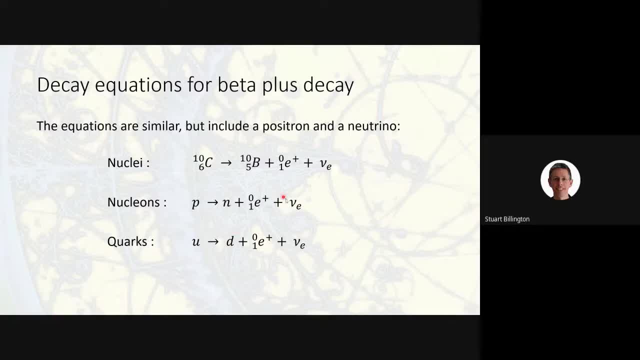 swap the up and the down round, and we've just changed these from leptons to anti-leptons, So the electron becomes an anti-electron and the anti-electron-neutrino becomes a full-fledged electron-neutrino. OK, 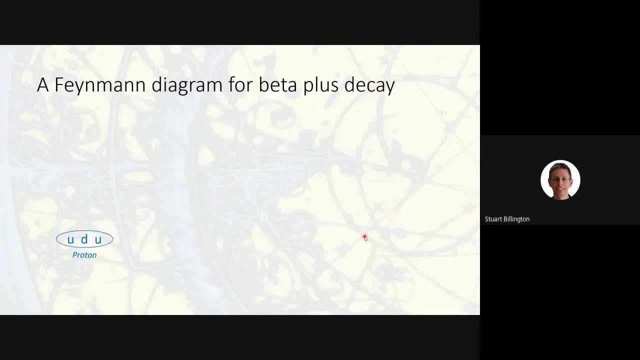 You might have had a go at the Feynman diagram. So there's the proton at the bottom, two ups and a down. The two up, The up and the down, carry on and do nothing at all, but the up decays. 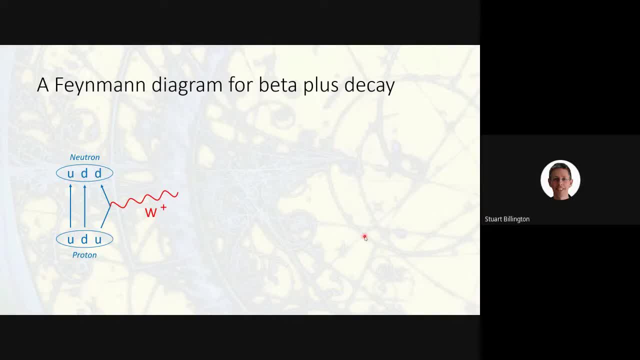 This time it's shed one positive amount of electric charge. So this time the charge carrier, the W, is carrying a positive amount of electric charge And, just as before, the W is an unstable particle and will decay. And when it does decay, 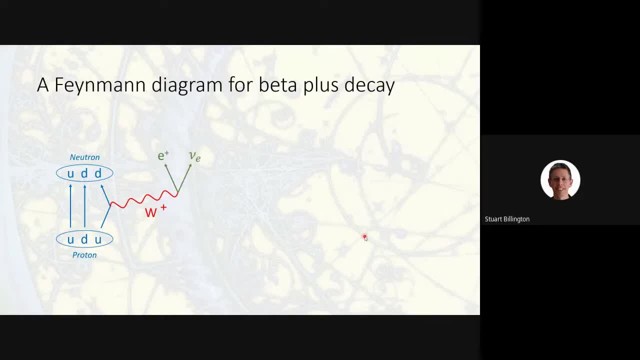 it decays into a lepton-anti-lepton pair Again. the Feynman diagram is not examinable, So if you didn't write that down, don't worry about it. OK, so I left you with the question of. 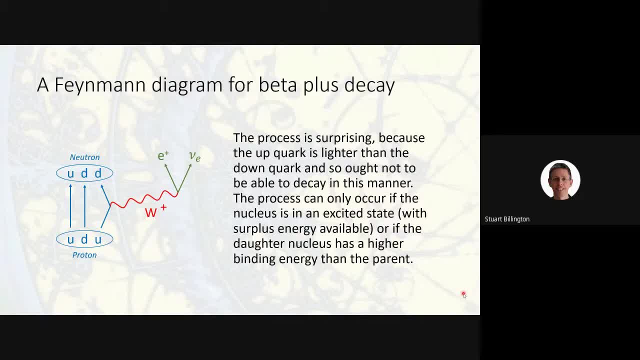 why is it surprising? And the reason it's surprising is because I said to you that beta-minus happens because the down is a heavy particle that can decay into a lighter one, which will be more stable. Well, what we have here is a light particle. 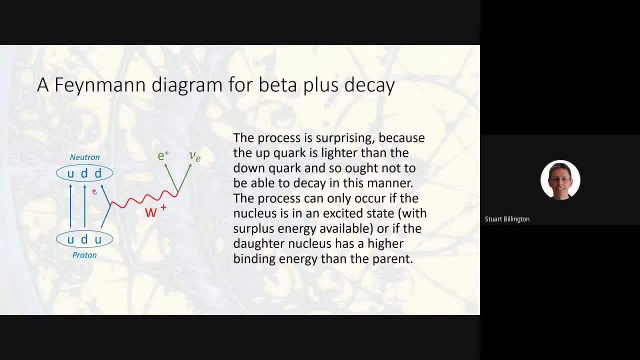 decaying into a heavier particle. In fact, this light quark the up is the lightest of all six quarks. it has the least mass of all of them. This quark, with the least mass of all, has managed to decay into a heavier down quark. 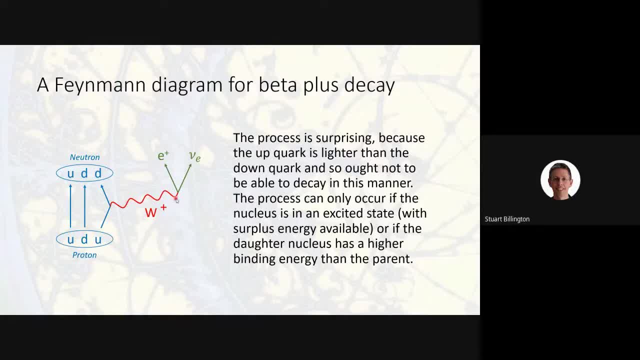 and a heavier W plus, Which begs the question of what kind of bank got robbed in the universe's energy scale that allowed this light particle to steal some mass from somewhere to create these two heavier particles. So the answer to why is it surprising is because this should be impossible. 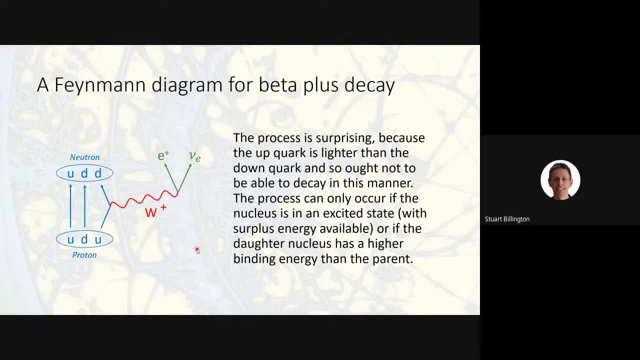 This goes against our conservation laws. And then you have to factor in that the real world is a little bit more complicated than A-level physics, And it's routinely the case that nuclei might exist. in excited states, Nuclear processes occur, which leaves the nucleons inside a nucleus. 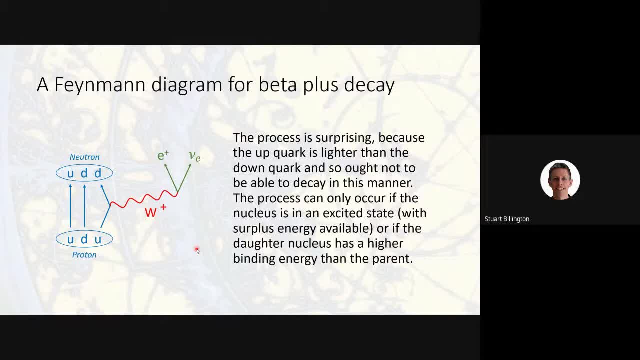 with more energy than they're supposed to have, And what has happened here is that the up hasn't used its mass energy to do this. The up has somehow found itself maybe in possession of a lot of potential energy from the strong nuclear force, or a lot of kinetic energy. 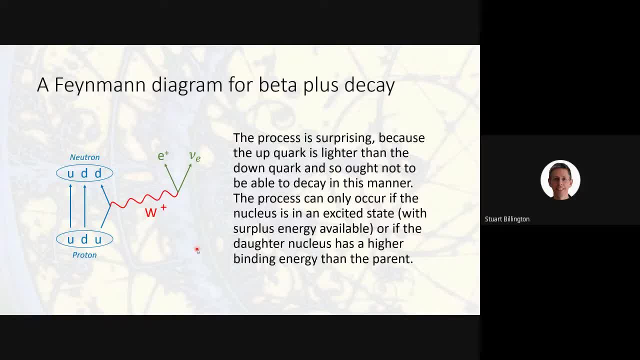 from some process that's occurred within the nucleus And the up has just got itself a little bag of energy that it has decided to invest in upgrading itself from a lighter up to a heavier down, And then it even had some leftover at the end. 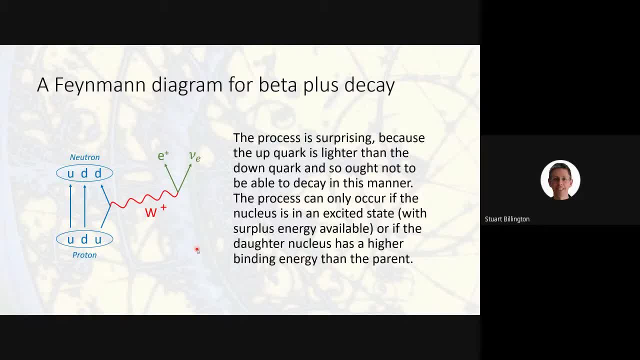 which it gambled away on a W plus particle. So sometimes this is possible because of excited states. But if you really want to make your head bend a little bit about the difference or the chain of events between cause and effect, it turns out actually that 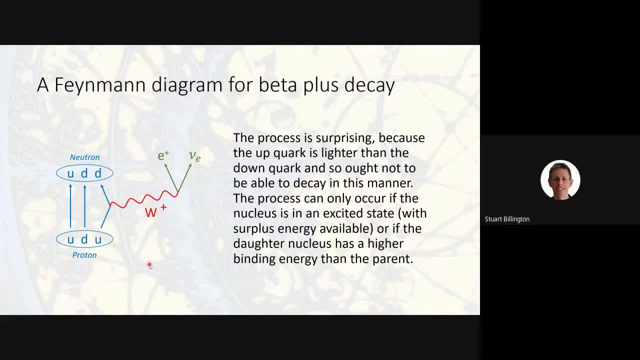 you need to take a more holistic view of beta plus decay and ask what happened to the nucleus as a whole when we swapped a proton for a neutron And what will have occurred if you go back to the binding energy per nucleon graph. is that the daughter nucleus? 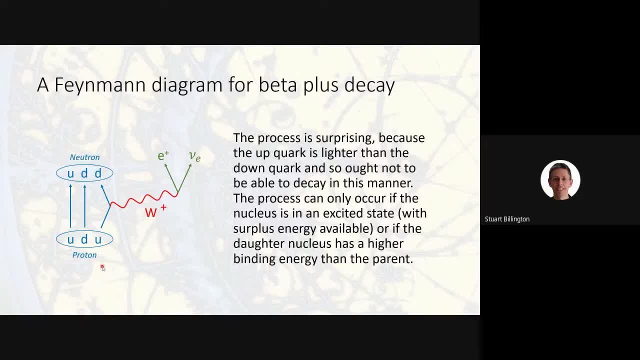 that has an extra neutron and one fewer proton. if you look the daughter nucleus up on the binding energy graph, you will discover that the daughter nucleus has a higher binding energy and therefore is more stable than the parent nucleus. And therefore, if it makes your head hurt enough, 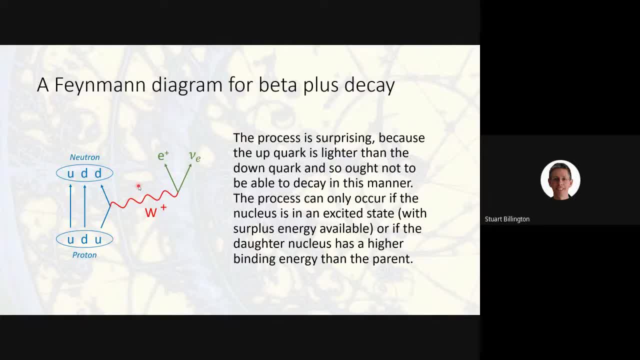 the decay occurred because the universe accepted that the outcome would have less energy at the end of the process, even though more energy was required during the process to make it occur. If you do chemistry, you'll be aware we've spoken before about enthalpy graphs. 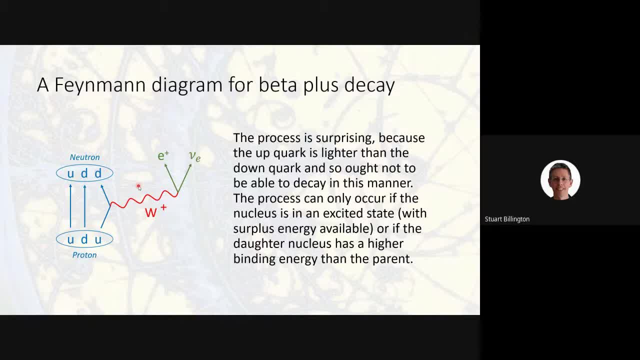 where there is an initial activation energy that needs to be overcome in order to produce a net gain from an exothermic reaction. Like when you set fire to carbon, you need to put a little bit of energy in to make it react with the oxygen. 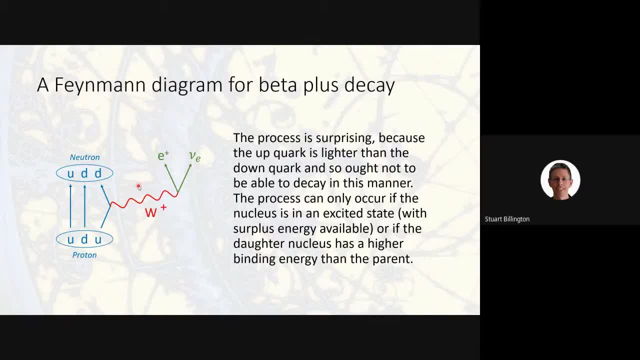 But when you do so far, more energy comes out from the reaction than what you put in to get it started. The analogy here is that the up borrowed a little bit of energy from the universe and made a decay equation take place that resulted in a net gain of energy. 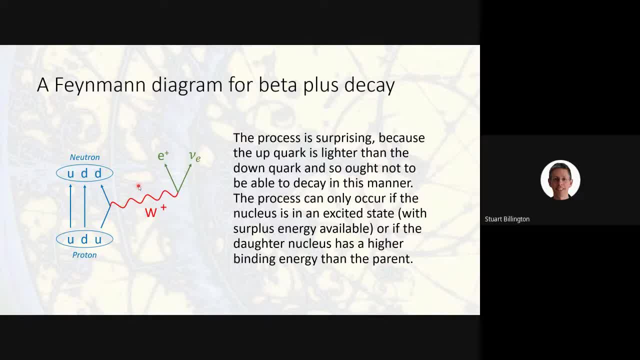 to the universe, paying back what was borrowed, and then some in interest as well. Quantum mechanics doesn't really pay much attention to the direction of the time arrow at a fundamental level, and it couldn't care less whether it is breaking cause and effect over very small time scales. 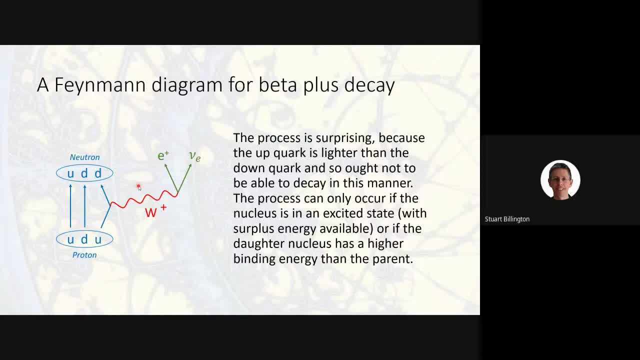 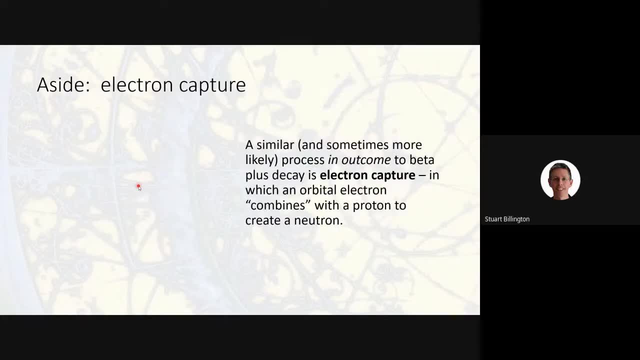 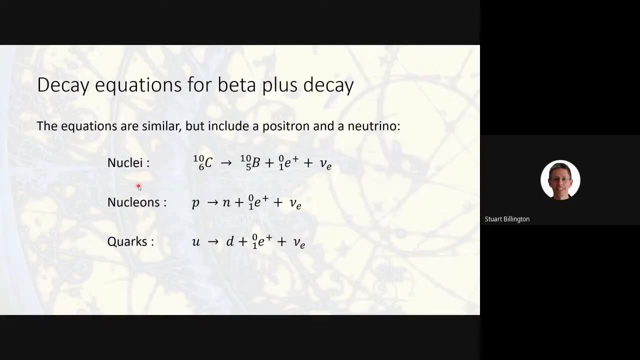 It's probably healthier not to think about it too much, otherwise you'll get a headache. Okay, last slide. Exactly the same equations, these equations. The effect would be the same if, instead of a proton emitting a positron, which, remember, requires a net amount of energy. 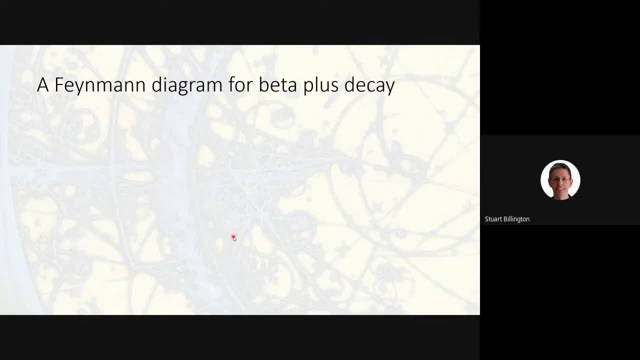 to be borrowed initially. What you can have instead is again thinking holistically. this positron is going to nip off into the universe and it will collide with an electron somewhere and it will annihilate. and this positron will disappear from the universe and it will take an electron with it. 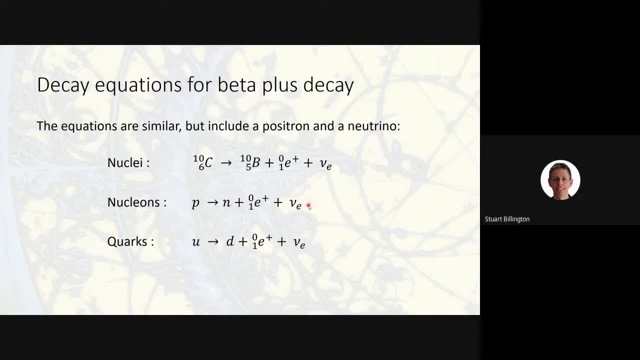 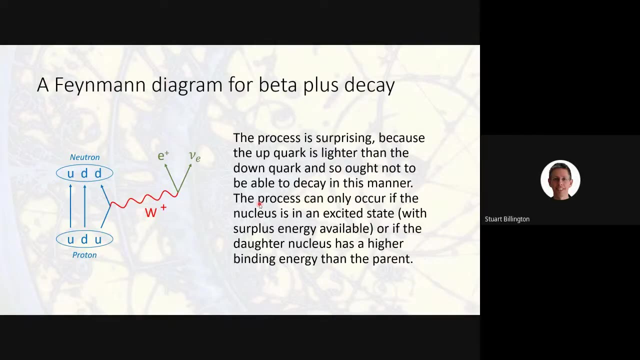 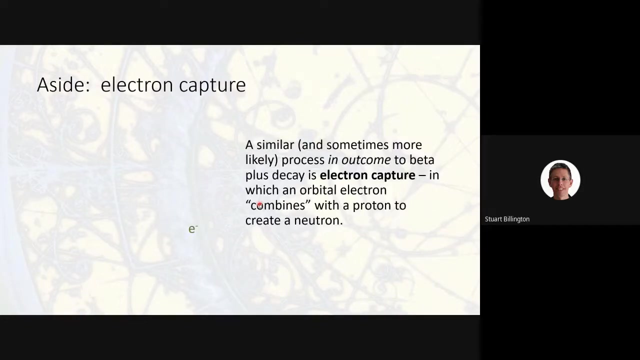 So, within moments of this decay, what will actually occur is that an electron will disappear from the universe when it annihilates with this positron. So in beta plus decay, the outcome eventually is the disappearance of an electron and in its place an electron neutrino. 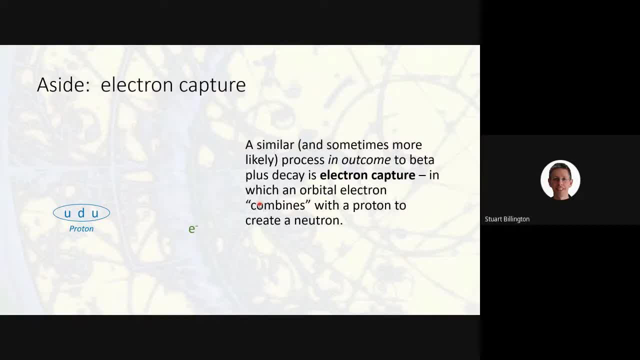 So we can actually consider a slightly more likely event, perhaps in a very large atom that has a lot of orbital electrons. You will remember from your chemistry that the orbitals of the electrons are fuzzy, smeared out probability zones and actually there is a non-zero probability. 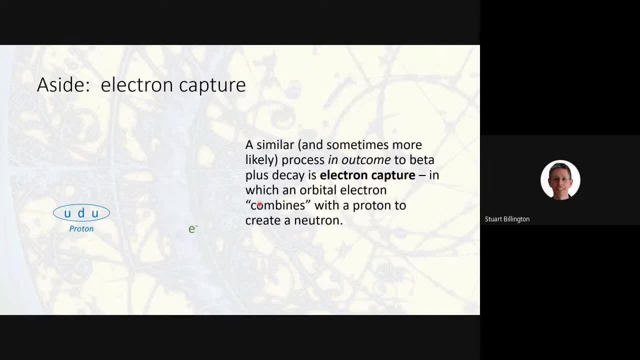 of an electron. So what we can do is we can actually consider an electron existing within the nucleus momentarily, and it is possible for an electron that accidentally trespasses into the nucleus to find itself interacting with a quark there. So an electron gets a little bit too close. 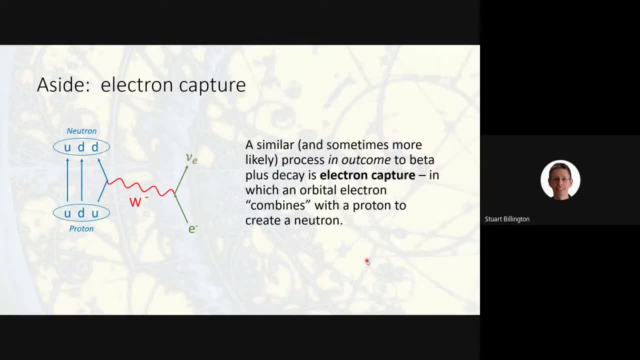 to an up quark and as it encounters the up quark, the electron decays into a neutrino and fires a decay particle, the W, at the up quark, and the up quark absorbs it and becomes the down quark. The process is different. 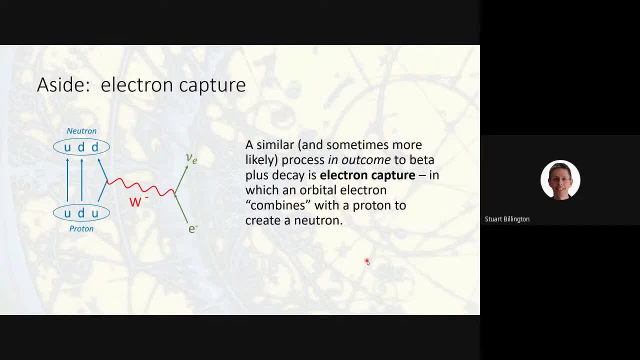 in terms of which order things happen in, but the outcome is the same: An up turned into a down, an electron ceased to exist and an electron neutrino began to exist. If you read enough about Feynman diagrams, you will realise that time is really not very important. 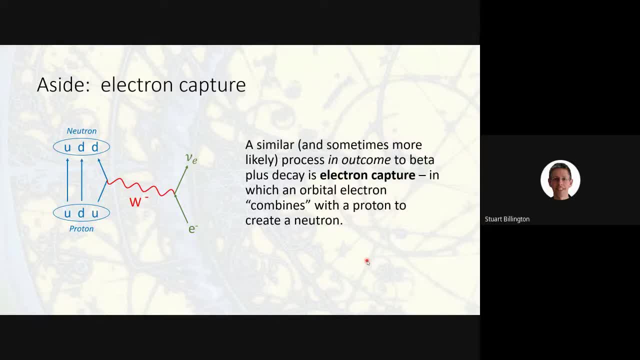 in the standard model and the order in which things happen really isn't that crucial. We really just like to ask: what was the state of affairs at the beginning? what was the state of affairs at the end? and in between, just shut up and calculate and don't worry too much.